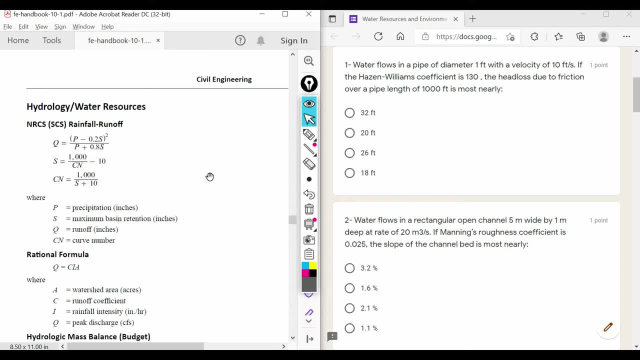 second, If the Heisen-Williams coefficient is 130, the head loss due to friction over a pipe length of 1000 feet is most nearly which of the following: So, in order to solve this problem, we need to use the Heisen-Williams formula, so which we can find by typing the weird formula, because 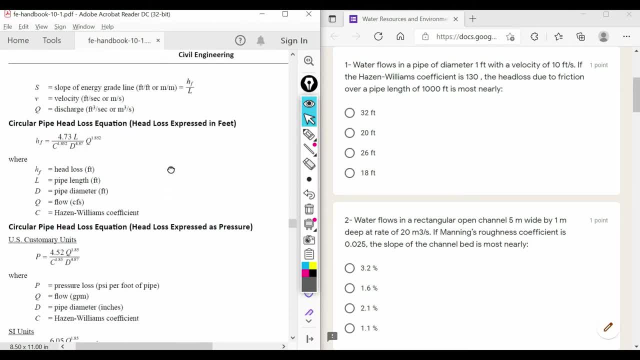 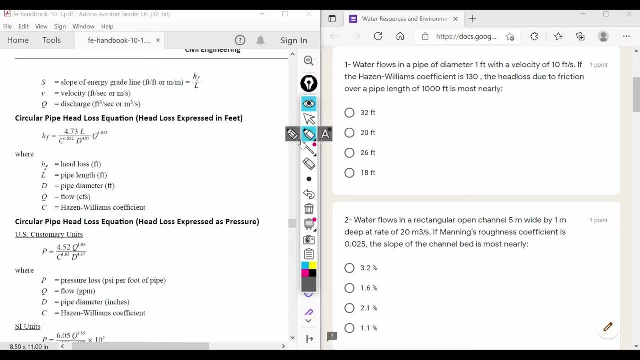 it comes after the weird formula in the hydrology section. So here is the, the formula we are looking for. so here is our formula and here our. our l is equal to 1000 feet, so we don't need to transform because all the units are expressed. 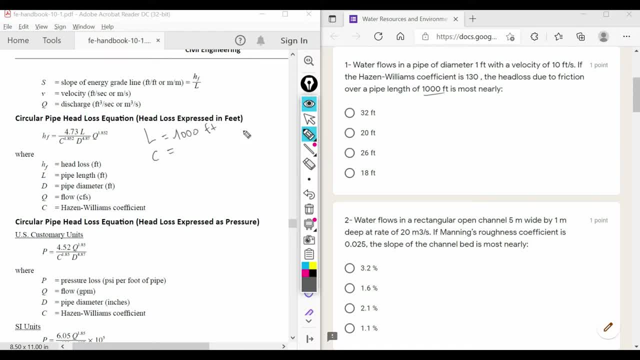 in feet here. so the c is equal to 130 and d, which is the diameter. pipe diameter is one foot. and finally we need to express the, the flow rate. so the flow is equal to the velocity multiplied by the section of the pipe. so here we have: the velocity is equal to v. 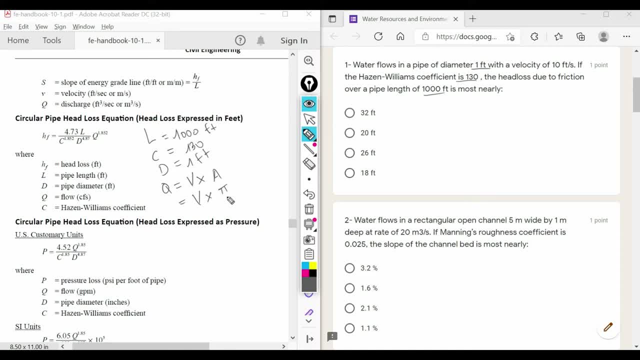 which is equal to 10, multiplied by the section, which is p over 4, multiplied by diameter square. so now, if we plug in the numbers, we'll have 4.73 multiplied by one thousandths over c, which is equal to 130, to the power of 1.852 times d, which is equal to one. 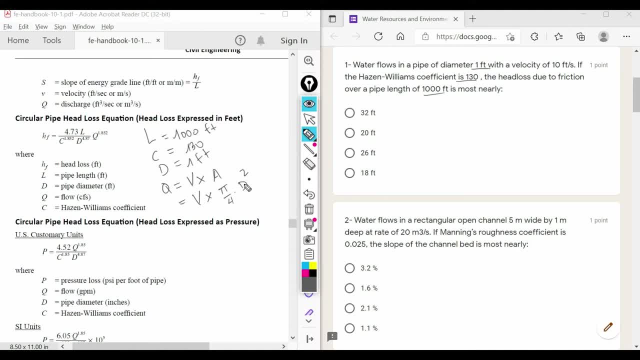 foot, feet, and finally we multiply the results by 10, multiply by p over 4, to the power of 1852. so, and the good answer is, uh, 26.13 feet, which is with the close to 26. so we choose this, this answer, here. and, by the way, if you want to have an idea about the coefficients, heisen williams. 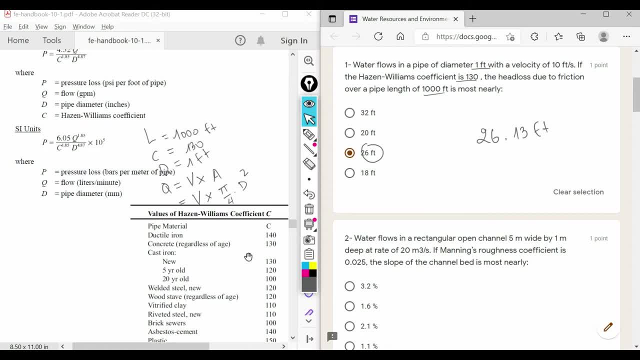 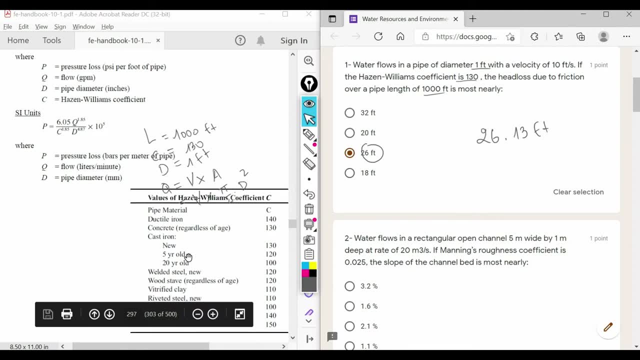 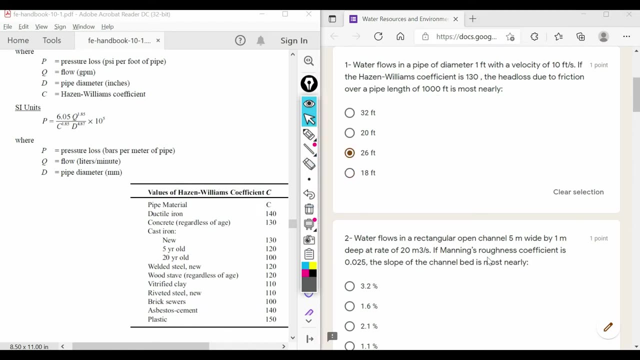 coefficients. there is a table here that gives you all you need in function of the property of the material or the pipe you are using. so let's move now to the second question. so the second question is about um manning's uh formula. so water flows in a rectangle, open channel five meter wide. 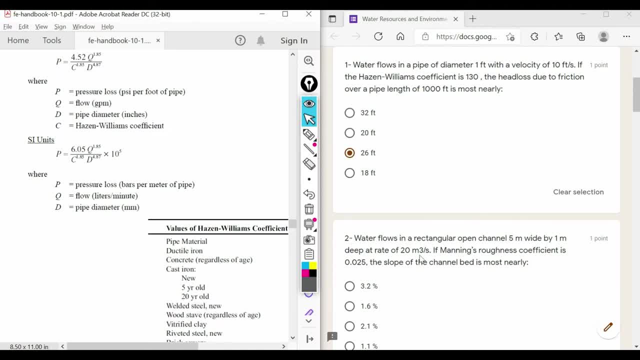 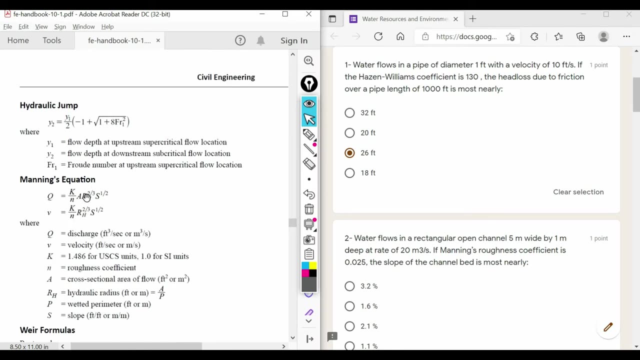 and one meter deep, at a rate of 20 cube meters per second. if money's roughness coefficient is 0.025, slope of the channel bed is most nearly which. so let's use the mining formula. so this is mining equations. you have two kind of equations. if you had the, if you have the, 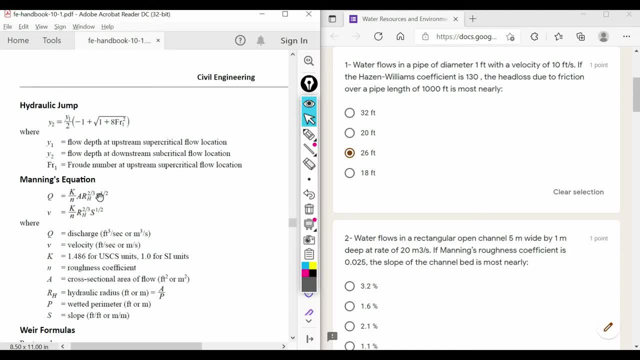 the discharge, you use this one. so here what we have. so let's analyze this questions. so here we have this. uh, okay, it's known because we'll use here the uh international system. so k will be equal to one and a is the area cross-sectional area of the flow, which is five. 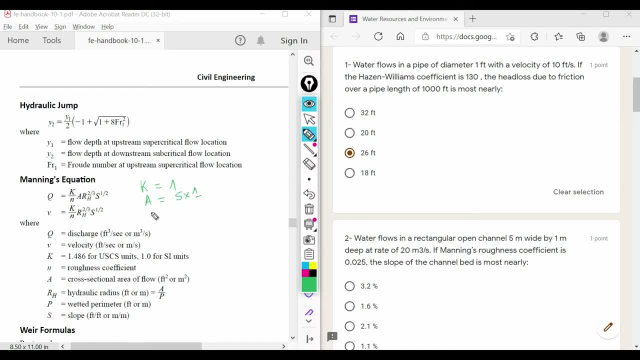 multiply by one, which is five meter squares, and here we have, uh, the hydraulic, uh radius, which is equal to the cross-section over the perimeter. but here you have to pay attention, because here we have a knotting channel. so we'll have a channel which is like this, okay, and we'll have the surface of the water. 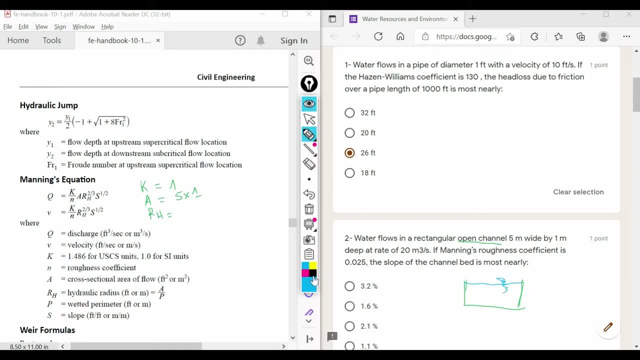 surface of the water. so here we'll have um five meters and here we'll have one meter. so the section is this. one section here is equal to five meters square. but the perimeter we are looking for order to calculate the hydraulic radius is the weighted perimeter. what is the weighted perimeter is the sum of the sides that. 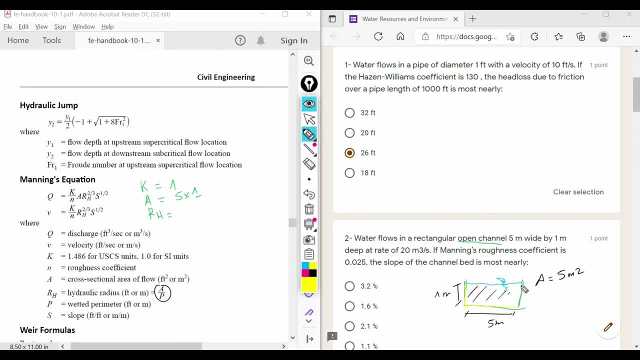 are weighted. so we have this side plus this side plus this side, so we have only three sides uh that constitute the widget, uh perimeter. so the good answer here for p will be five plus one plus one, which is equal to five plus one plus one which is equal to seven, and not five plus one multiplied by. 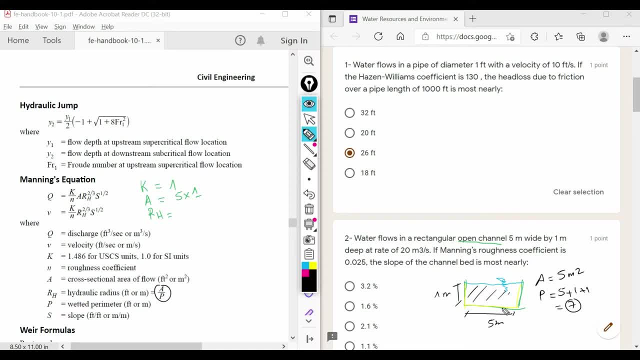 two, which is equal to twelve. so it's very important to calculate the p in order to have the good value for rh. so the hydraulic radius will be here, five over seven, and finally we need s. so this is what we are looking for in this exercise: what is most nearly slow. so either you can calculate the velocity, 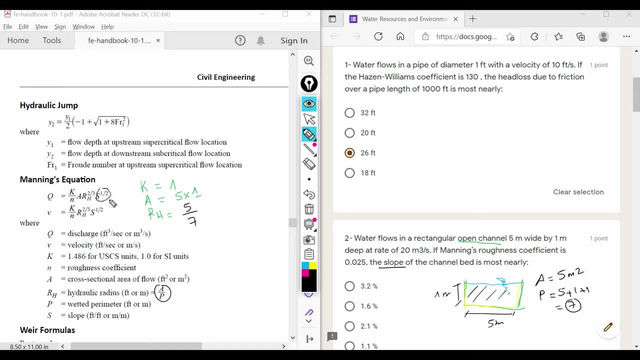 or you can use your calculator, the feature of your calculator, in order to uh, to find s directly, or you can just move this, uh, these values, to this side in order to to find s. so i will show you the feature in in casio, uh, in casio. so give me one minute to. so where is the emulator of the casio? 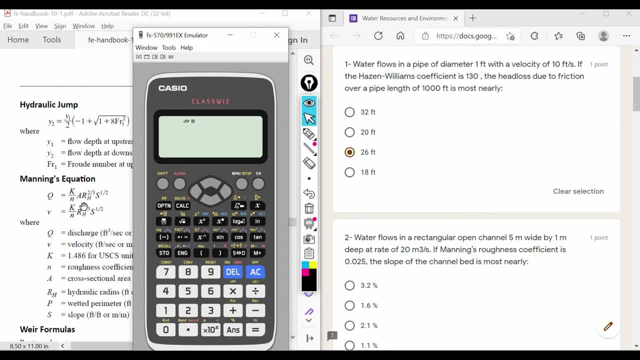 um, let's just type this uh equation and i will show you the feature. you don't need to uh to find s as function of all this value, you have just to type this equation. so we have. we have here q equal to 20, so 20 alpha equal, and the k is equal to 1 over the roughness coefficient or mining coefficient. 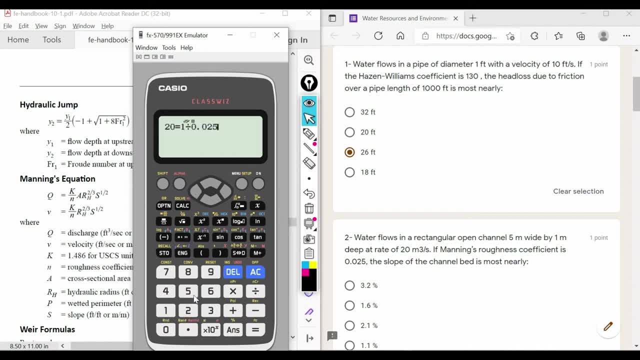 is zero point zero, 25 multiplied by the area, which is 5 multiplied by 1, so 5 multiplied by the hydraulic radius that we calculated. so it's uh 5 over 7. to this power here, 2 over 3, and multiply by our s? s in that case is x in order to solve the function. so we call this x. 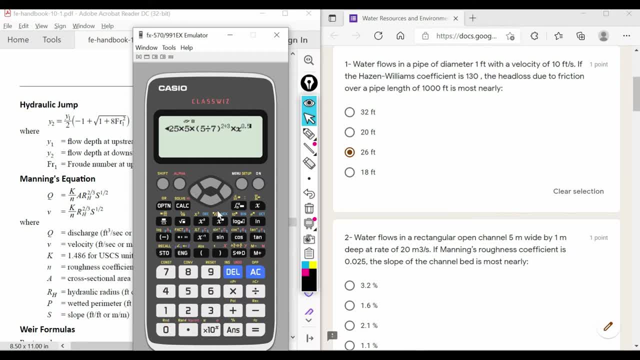 and to the power of 0.5. now the second step is just to click shift, solve and equal and you will have your value, which is 0.015, and 0.015 uh 6, it's equal to 0.016, which is 1.6 percent. 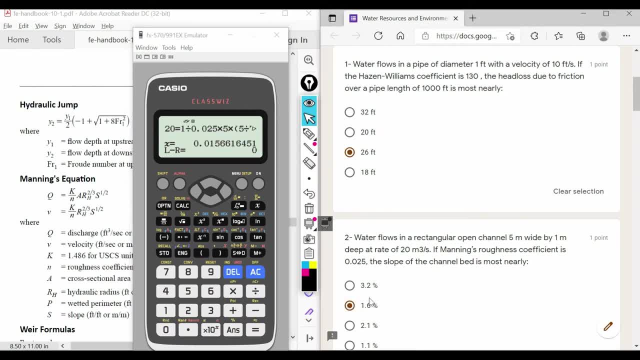 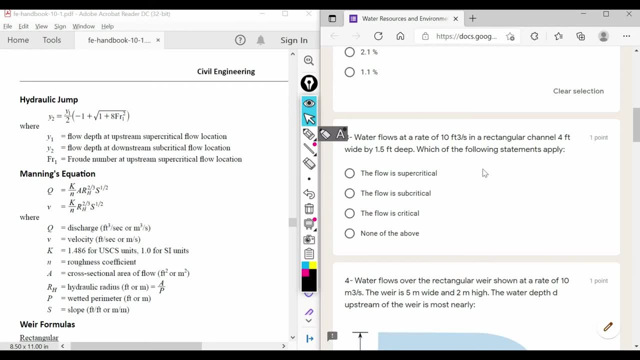 so the curse answer is this one, so let's move to question number three. so for question number uh three, we have water flows at rate of 10 cubic feet per second in a rectangular channel 4 feet wide by 1.5 feet deep. which of the following? 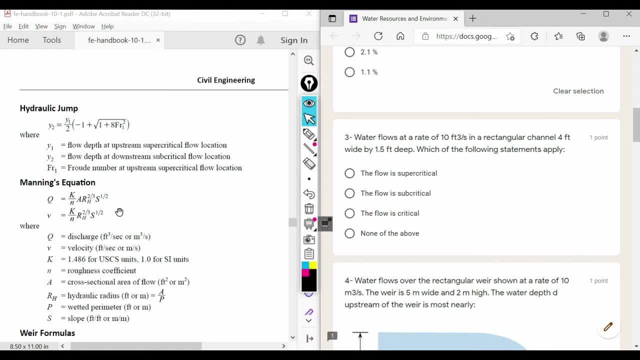 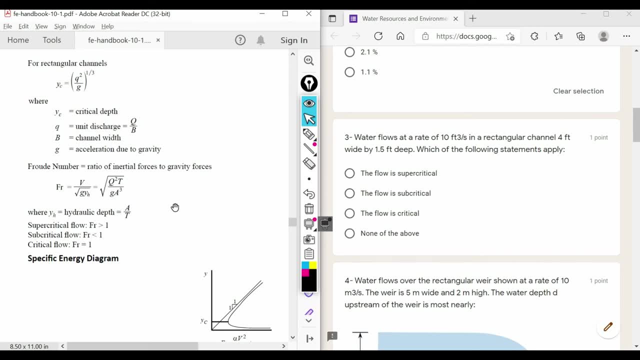 statements apply. so here we have the type of flow: subcritical, critical, etc. you have to use this food number in order to qualify the flow. so if the fruit number is more than one, the flow is super critical. if it's less than one, the flow is subcritical. and finally, if it's equal. 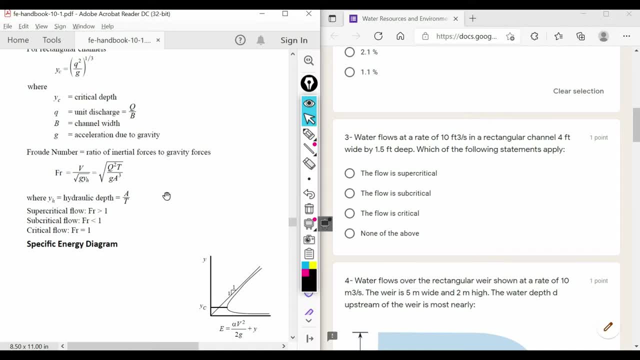 to one: the flow is critical. so here is the formula. let's try to use the information we have, using this formula in order to find the good answer. so here we have this formula here. so Q is the flow, the flow rate which is equal to 10 cubic foot per second, and T, let's, let's. 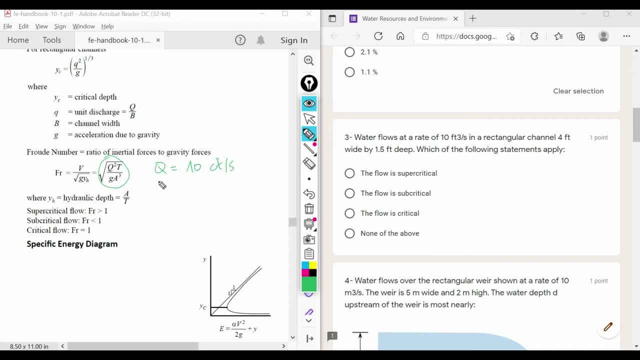 talk first about j. J is the acceleration of gravity. so if we use the US units we have use 32 points, two or four, I don't remember, but the precision is not very important, so you have to check. maybe 32.2 or 32.4. you can find this value at 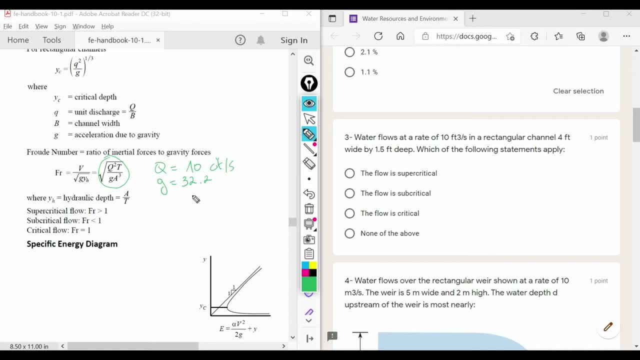 the beginning of the book where you have lots of units and units that conversions, etc. so here, a is equal to the cross-section, which is equal to 4 multiplied by 1.5. so in that case is 4 x 1.5, 1.5. and finally, the T. T is defined as: 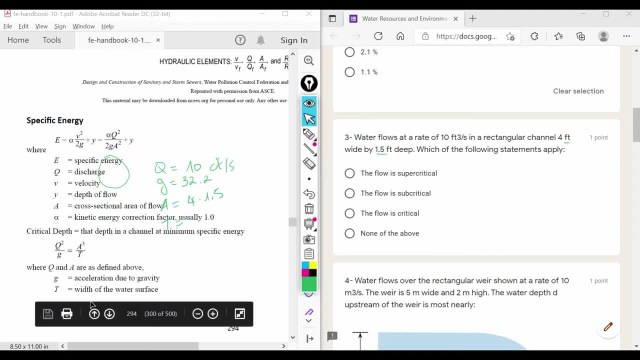 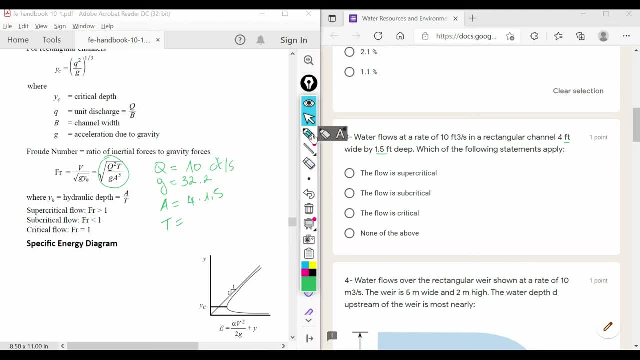 water surface, the width of the water water surface, the width of the water surface. so we have rectangle channel surface. so we have rectangle channel surface. so we have rectangle channel with 4 feet wide and 1 point deep and with 4 feet wide and 1 point deep and 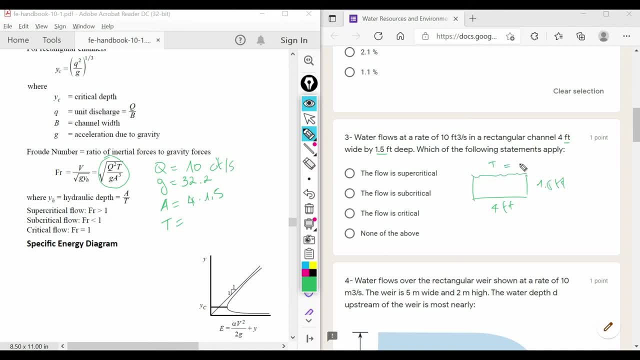 with 4 feet wide and 1 point deep. and here is the water surface. so T is equal. here is the water surface, so T is equal. here is the water surface. so T is equal to 4 in our case. so, finally, if we plug, to 4 in our case. so, finally, if we plug, 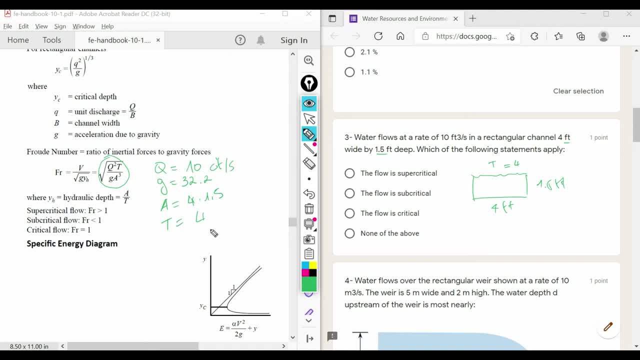 to 4 in our case. so finally, if we plug and and and, check we have find square root of 10. check we have find square root of 10. check we have find square root of 10. square multiply by 4 over 32.2 or 4. 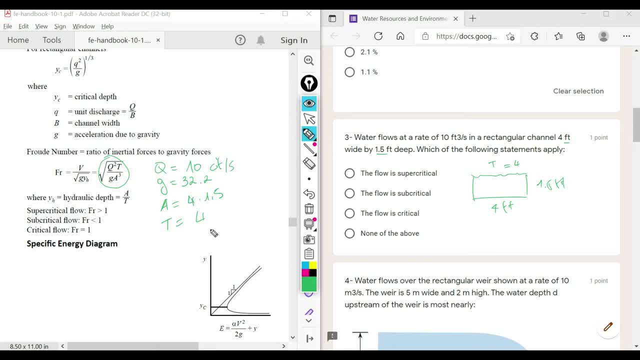 square multiply by 4 over 32.2 or 4. square multiply by 4 over 32.2 or 4. please check. multiply by 4: 1.5 to the. please check: multiply by 4: 1.5 to the. please check. multiply by 4- 1.5 to the third power, and we find 0.24, which is. 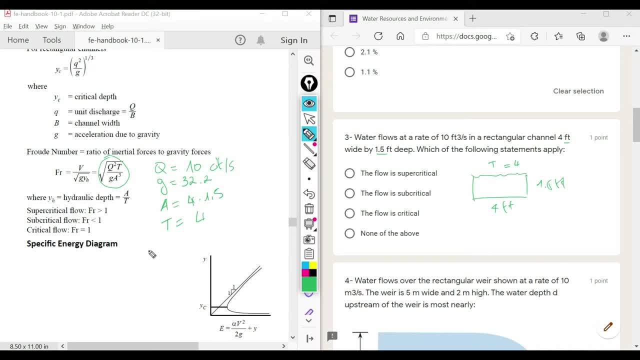 third power and we find 0.24, which is third power, and we find 0.24, which is less than less than less than this value here, so we have fruit number. this value here, so we have fruit number, this value, here so we have fruit number, is 0.24, which is less than 1, and the good. 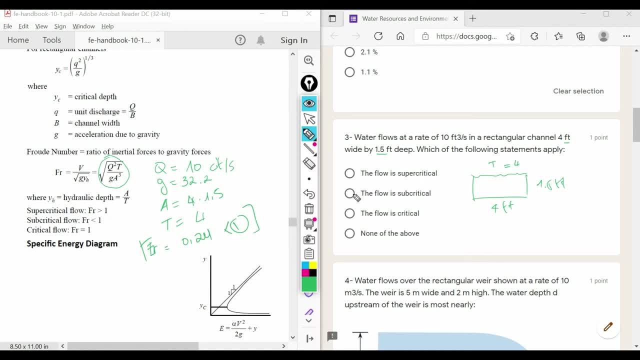 is 0.24, which is less than 1, and the good is 0.24, which is less than 1, and the good answer is the flow is subcritical. so answer is: the flow is subcritical. so answer is: the flow is subcritical. so let's move to the next question. so 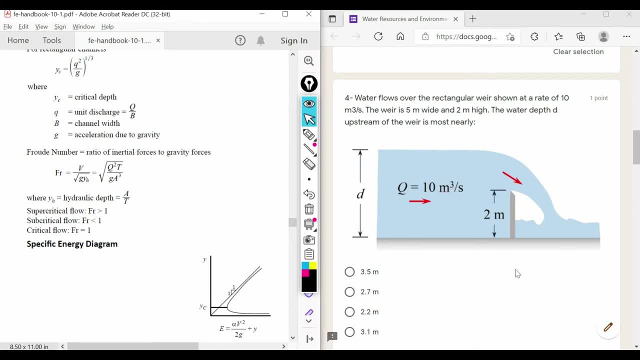 let's move to the next question. so let's move to the next question. so question number 4 is about the wheel. question number 4 is about the wheel. question number 4 is about the wheel formula. so water flows over the formula. so water flows over the. 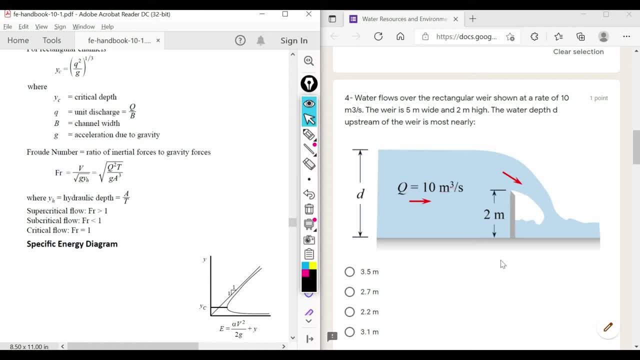 formula. so water flows over the rectangular. we've shown at a rate of 10 rectangular. we've shown at a rate of 10 rectangular. we've shown at a rate of 10 cubic meter per seconds. the wheel is cubic meter per seconds. the wheel is cubic meter per seconds. the wheel is 5 meter wide. so let's do so. here is the. 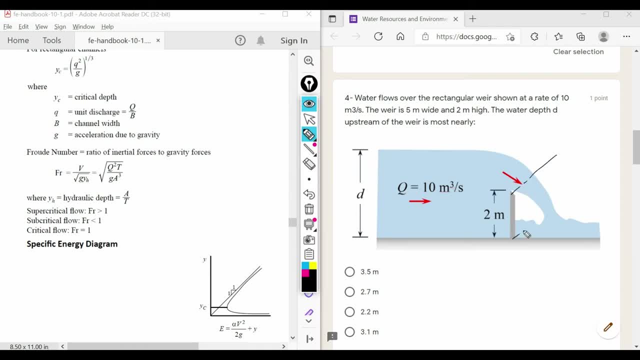 5 meter wide, so let's do so. here is the 5 meter wide, so let's do so. here is the height of the weir, and let's imagine height of the weir. and let's imagine height of the weir, and let's imagine that it's like this. so the this is the. 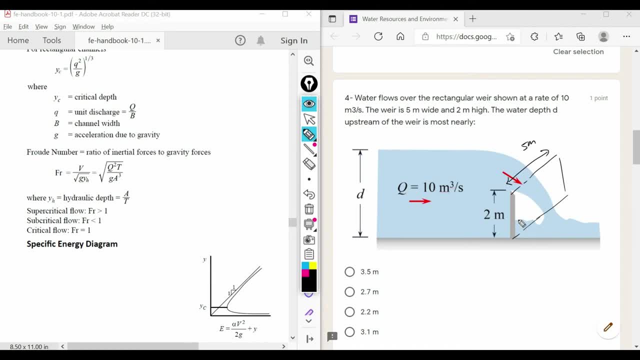 that it's like this, so the. this is the. that it's like this, so the. this is the width of the weir. it's 5 meter, so it's 2 width of the weir. it's 5 meter, so it's 2 width of the weir. it's 5 meter, so it's 2 meter height, high and 5 meter wide. and 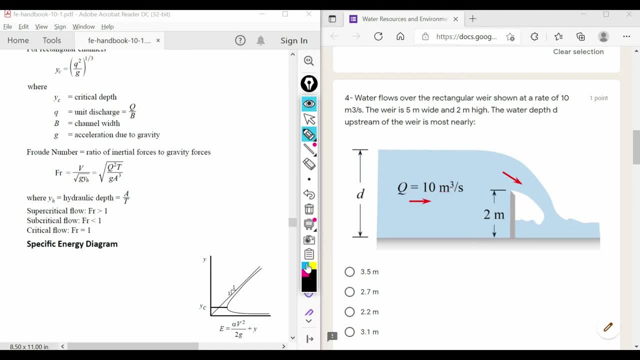 meter height, high and 5 meter wide, and meter height, high and 5 meter wide, and we are looking to for to calculate this. we are looking to for to calculate this. we are looking to for to calculate this value here, which is D, and what the value here, which is D, and what the. 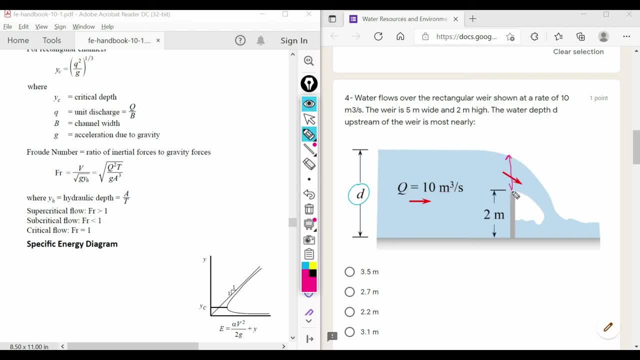 value here, which is D, and what the handbook formula gives us is this height handbook formula gives us. is this height handbook formula gives us: is this height? here, let's call it height H. so we know. here, let's call it height H. so we know. here, let's call it height H. so we know that the handbook formula gives us this. 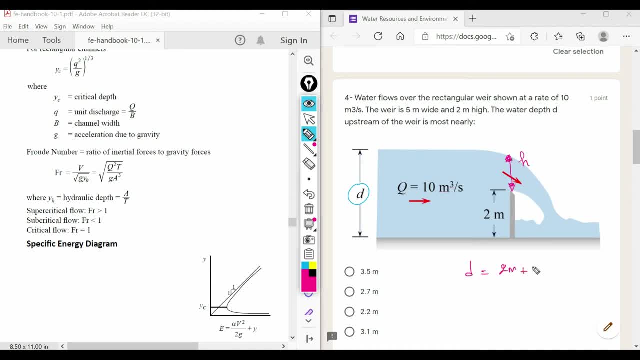 that the handbook formula gives us this, that the handbook formula gives us this: and D will be 2 meters plus H. now let's. and D will be 2 meters plus H. now, let's. and D will be 2 meters plus H. now, let's look for the handbook formula, so let's. 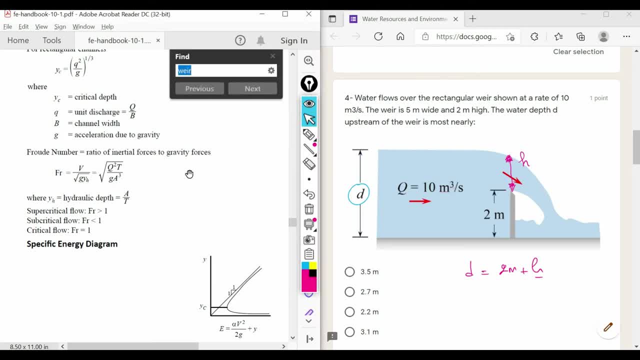 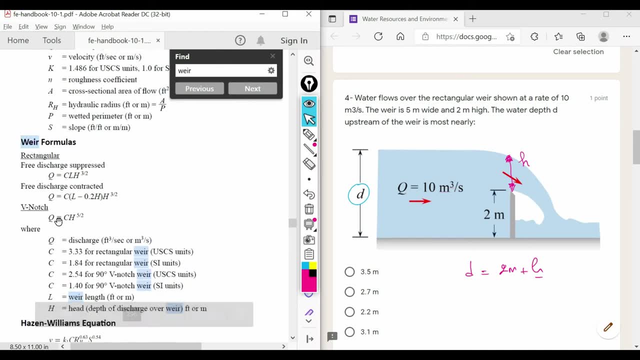 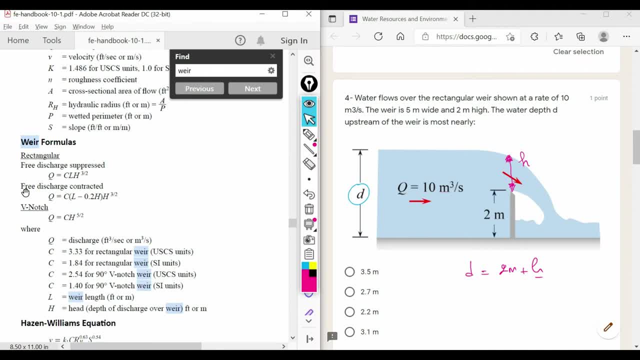 types. so we have the rectangle and the types. so we have the rectangle and the V notch and here we have a rectangular V notch, and here we have a rectangular V notch, and here we have a rectangular and we have, we have to use the first and we have, we have to use the first. 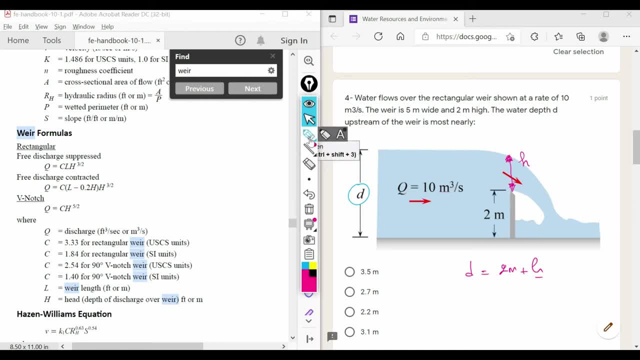 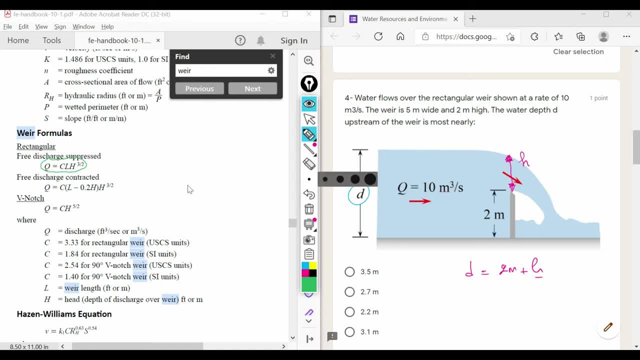 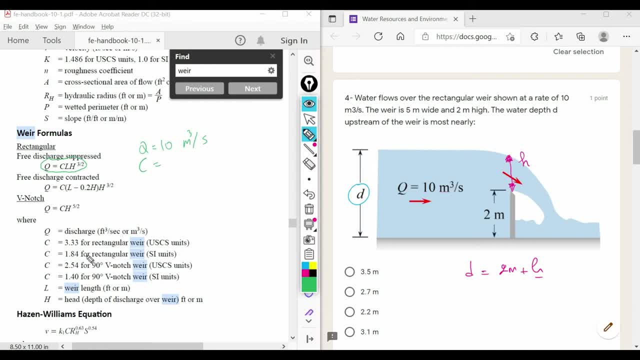 cube per second. C is a coefficient that depends of the units who are using here. depends of the units who are using here. depends of the units who are using here. so we are using a rectangular weir with. so we are using a rectangular weir with. so we are using a rectangular weir with international system. so C will be 1.8. 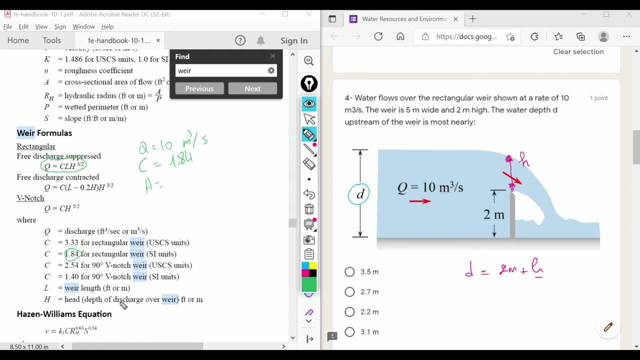 international system, so C will be 1.8 international system, so C will be 1.8 war, and H is the head or depth of this war. and H is the head or depth of this war and H is the head or depth of this charge over weir. so that's why H is from. 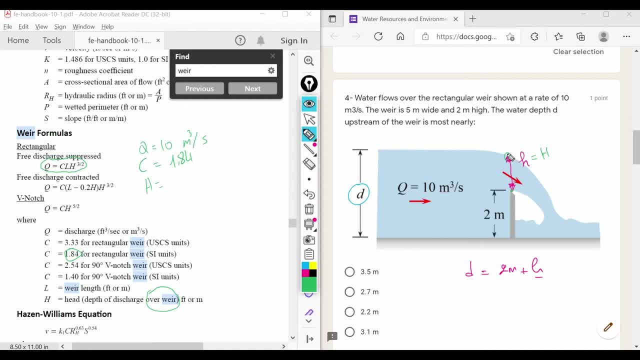 charge over weir. so that's why H is from charge over weir. so that's why H is from the height highest point of the weir to the height highest point of the weir to the height highest point of the weir to the highest point of the discharge. so 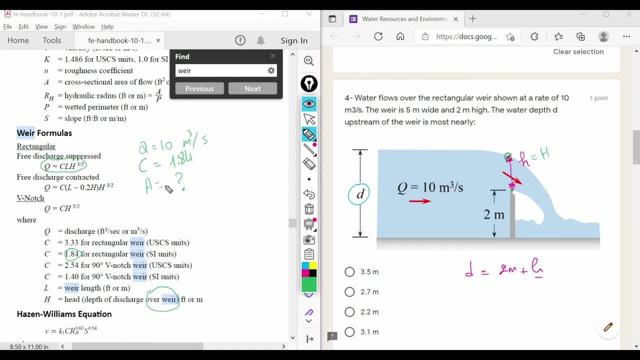 the highest point of the discharge, so the highest point of the discharge. so here is not now so you can use. of course here is not now, so you can use. of course here is not now so you can use. of course. you can try to express H as the. 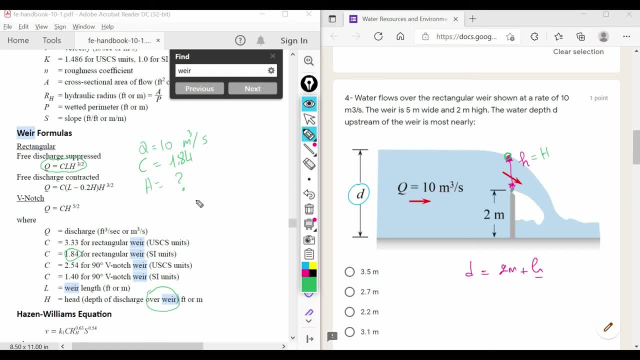 you can try to express H as the. you can try to express H as the function of QCL, or use the feature of your function of QCL, or use the feature of your function of QCL, or use the feature of your calculator. so let's use it in order. 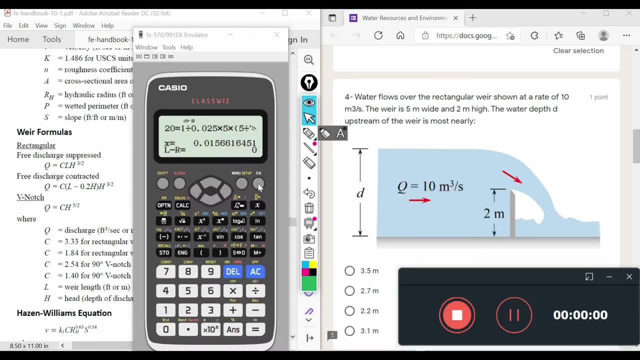 calculator, so let's use it in order. calculator, so let's use it in order to find the value of H. okay, so let's use to find the value of H. okay, so let's use to find the value of H. okay, so let's use the. so we have Q which is equal to 10, 10. 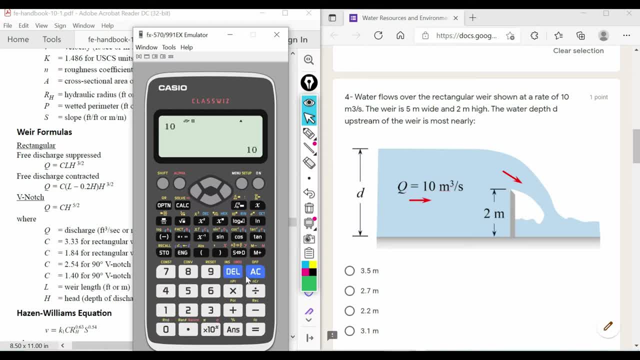 the, so we have Q which is equal to 10, 10, the, so we have Q which is equal to 10, 10. 10 is equal to- I'm sorry, 10 alpha equal 10 is equal to- I'm sorry. 10 alpha equal 10 is equal to- I'm sorry. 10 alpha equal to C, which is 1 point 8 for multiplied. 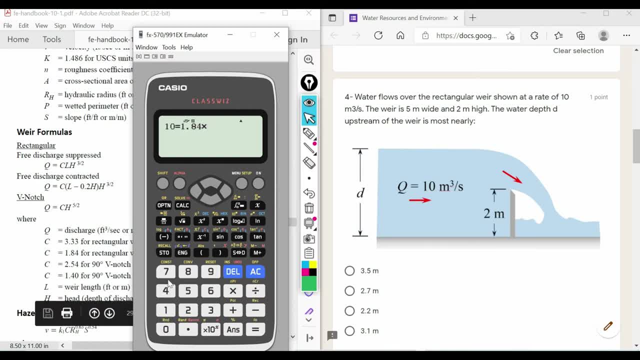 to C, which is 1 point 8 for multiplied to C, which is 1 point 8 for multiplied by L. L Heath is the weir length, but the by L Heath is the weir length, but the by L Heath is the weir length, but the weir length is the, actually the width of. 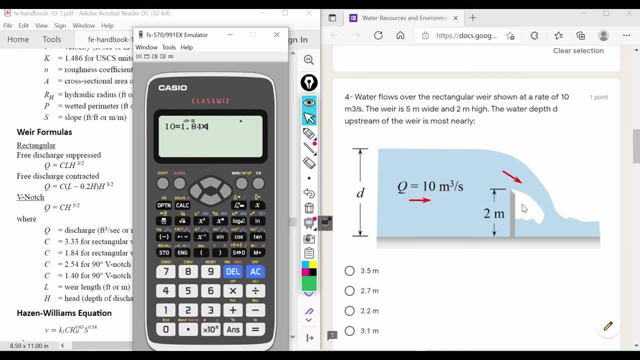 weir. length is the actually the width of weir. length is the actually the width of the weir. so the weir has two: the weir. so the weir has two: the weir. so the weir has two dimensions: the height and other dimensions. dimensions: the height and other dimensions. dimensions: the height and other dimensions, which is the the width and of. 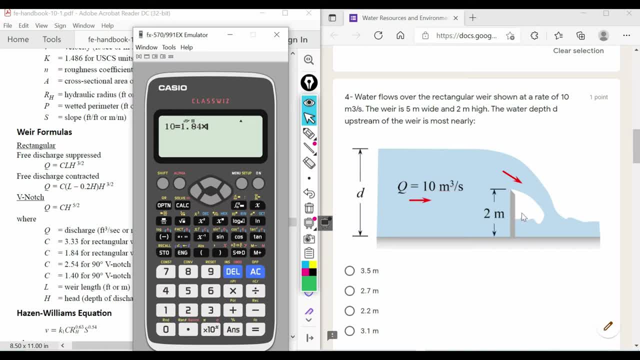 which is the the width and of which is the the width. and, of course, here we are not talking about the the course, here we are not talking about the the course. here we are not talking about the the depth or the thickness of the weir. depth or the thickness of the weir. 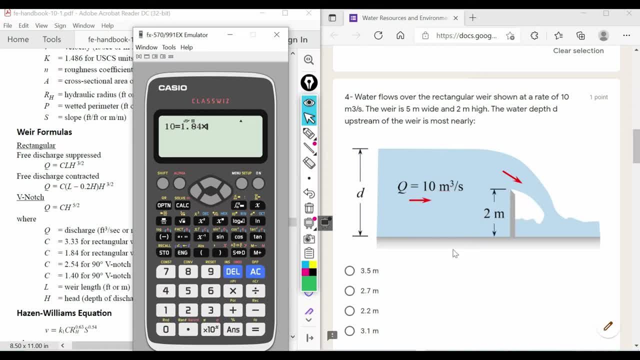 depth or the thickness of the weir. so we have the only to wear box height. so we have the only to wear box height. so we have the only to wear box height and the width. so the left, the width and the width. so the left, the width and the width. so the left, the width left here, which is the width in our 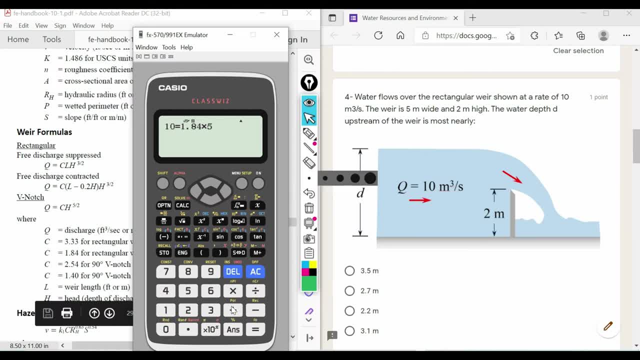 left here, which is the width in our left here, which is the width in our exercise, is equal to 5 x x, which is our exercise, is equal to 5 x x, which is our exercise, is equal to 5 x x, which is our, our H. so X to the power of 3 over 2. so 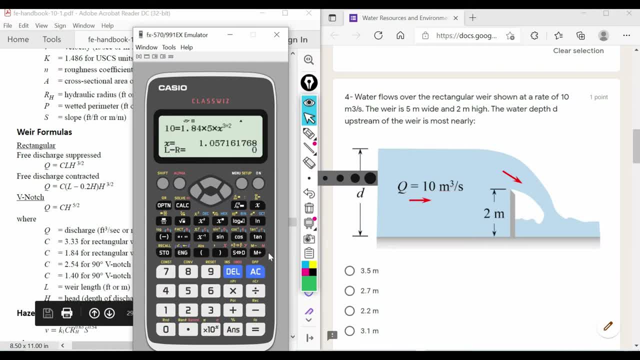 our H so X to the power of 3 over 2, so our H so X to the power of 3 over 2. so shift solve and our value here is 1.06. shift solve and our value here is 1.06. shift solve and our value here is 1.06. so let's write it down here, so H equals. 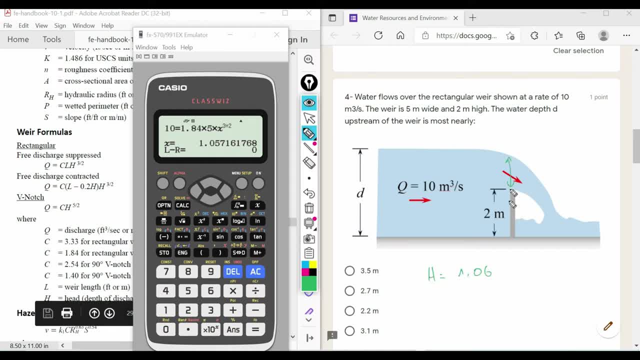 so let's write it down here: so H equals. so let's write it down here: so H equals 1.06, which is this value 1.06, which is this value, 1.06, which is this value here. so finally, D will be equal to 2 plus. 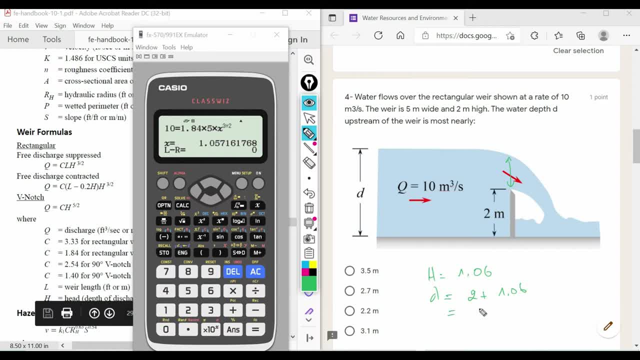 here. so finally D will be equal to 2 plus here, so finally D will be equal to 2 plus 1.06, which is equal to 3.06, which is 1.06, which is equal to 3.06, which is 1.06, which is equal to 3.06, which is closely equal or approximately equal to. 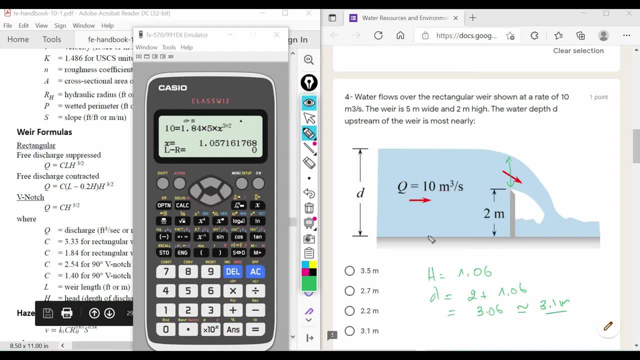 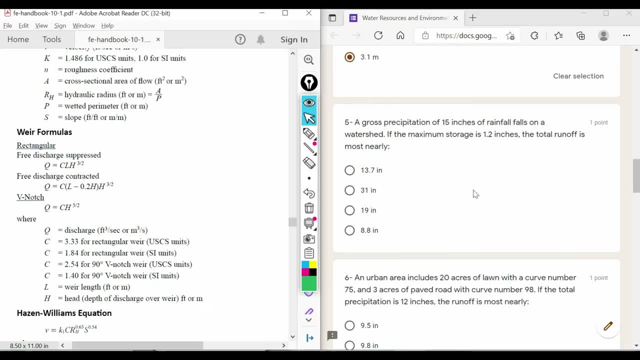 closely equal or approximately equal to closely equal or approximately equal to 3.1 meters, and a good answer here is D, 3.1 meters, and a good answer here is D, 3.1 meters, and a good answer here is D. so let's move to the next question. so 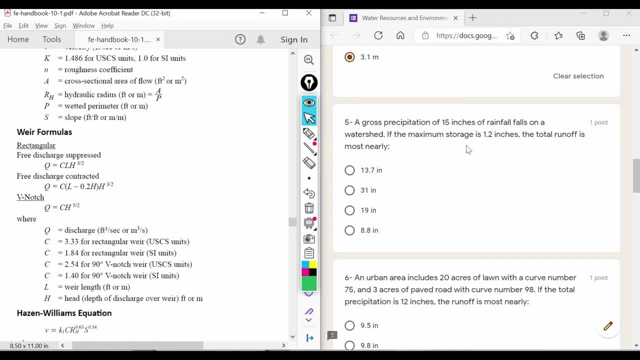 so let's move to the next question. so so, let's move to the next question. so, question number 5: a gross precipitation. question number 5: a gross precipitation. question number 5: a gross precipitation of 15 inches of rainfall falls of. of 15 inches of rainfall falls of. 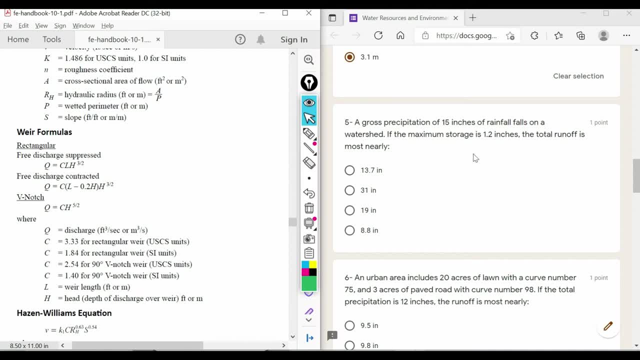 of 15 inches of rainfall falls of on a watershed. if the maximum storage is on a watershed. if the maximum storage is on a watershed. if the maximum storage is 1.2 inches, the total runoff is most. 1.2 inches. the total runoff is most. 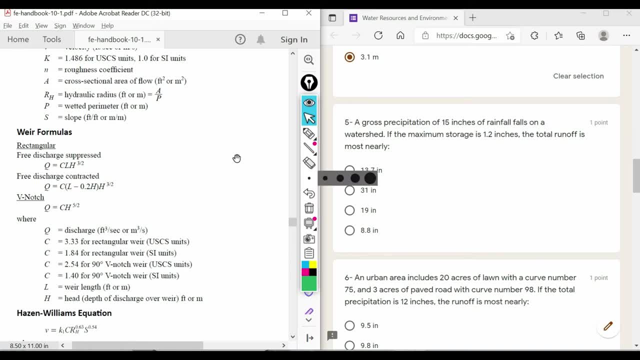 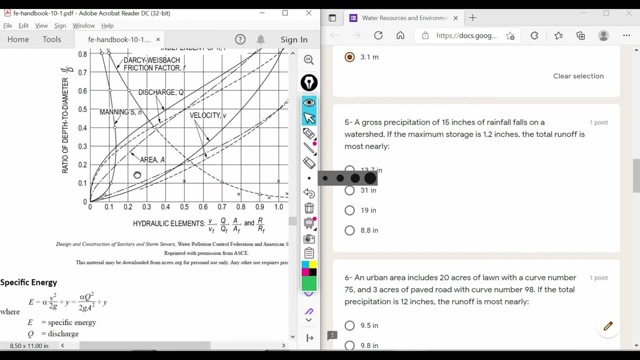 1.2 inches. the total runoff is most nearly which. so here we will use the nearly which. so here we will use the nearly which. so here we will use the runoff formulas that are at the beginning, runoff formulas that are at the beginning, runoff formulas that are at the beginning of the of the of this section. so let's. 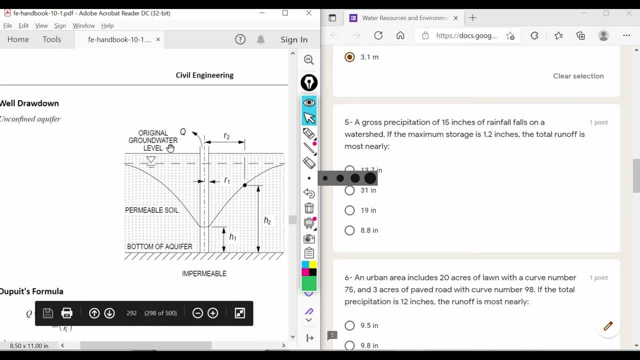 of the of this section, so let's of the of this section, so let's move back to to the beginning of the move, back to to the beginning of the move, back to to the beginning of the section. here we are, so, here we have the section. here we are, so here we have the. 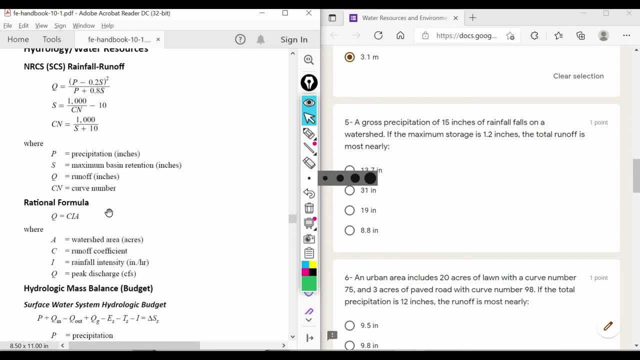 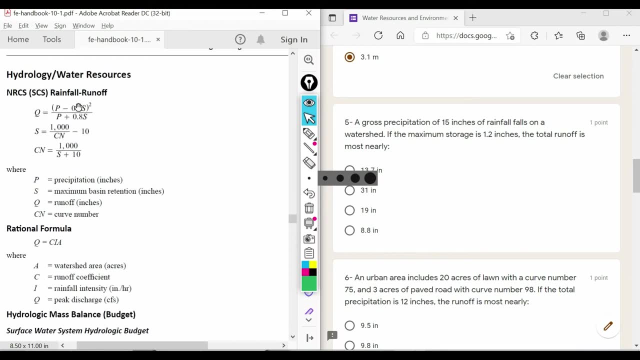 section. here we are. so here we have the rainfall formulas, we have two rainfall formulas, we have two rainfall formulas, we have two formulas to use the rational formula and formulas to use the rational formula and formulas to use the rational formula. and this on RCS, rainfall, runoff formula. so 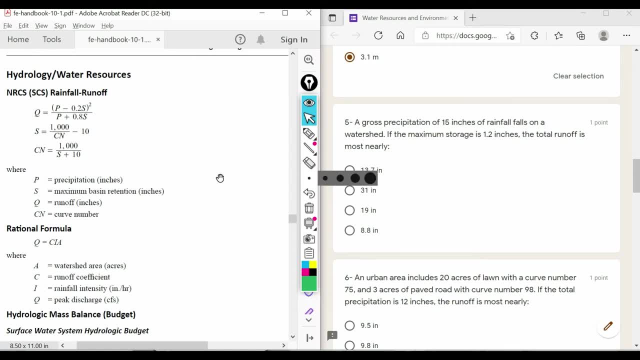 this on RCS rainfall runoff formula. so this on RCS rainfall runoff formula. so here we are given the storage. so so here we are given the storage. so so, here we are given the storage. so so what's given here is the storage, and of what's given here is the storage and of. 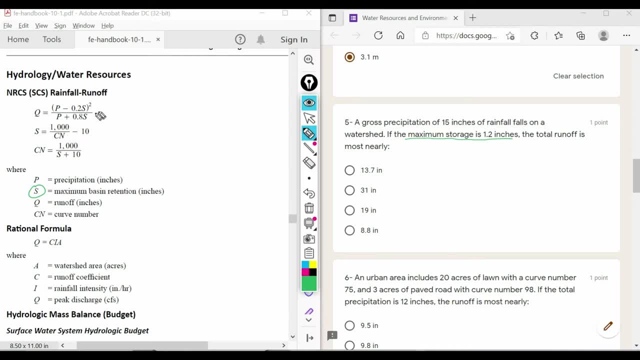 what's given here is the storage, and of course we use this formula here. so here, course we use this formula here. so here, course we use this formula here. so here is the formula I'm talking about. so is the formula I'm talking about. so is the formula I'm talking about. so Q is, and now, and in this formula is: 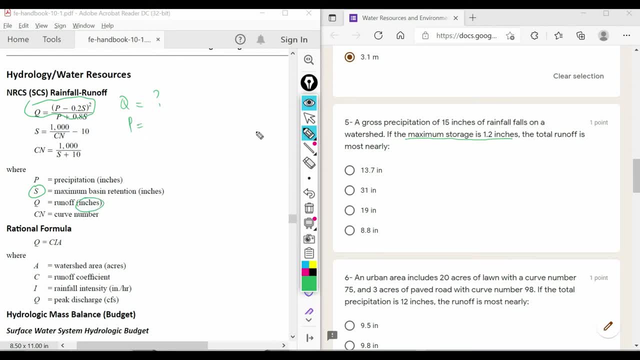 Q is and now, and in this formula is: Q is and now, and in this formula is expressed in inches: P is equal to 15. expressed in inches, P is equal to 15. expressed in inches, P is equal to 15 inches and S is equal to 1.2 inches. so 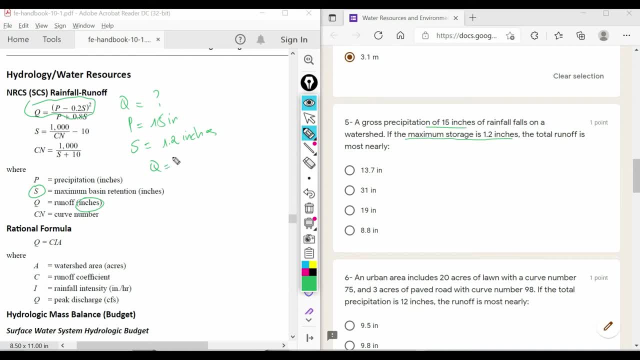 inches and S is equal to 1.2 inches. so inches and S is equal to 1.2 inches. so plug-and-check Q is equal to 15 minus plug-and-check Q is equal to 15 minus plug-and-check Q is equal to 15 minus 0.2 x 1.2. to the power second power over: 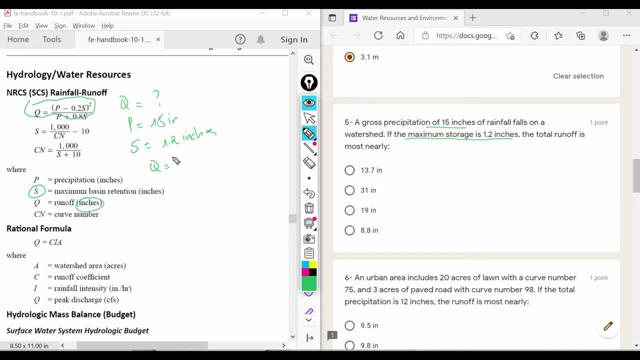 0.2 x 1.2 to the power. second power over 0.2 x 1.2 to the power. second power over 15 plus 0.8 multiplied by 1.2, which is 15 plus 0.8 multiplied by 1.2, which is: 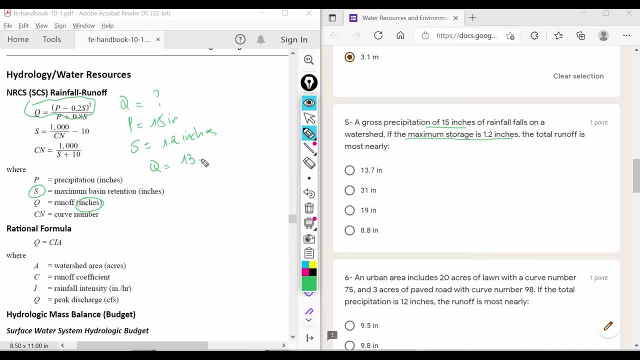 15 plus 0.8 multiplied by 1.2, which is equal to 13 points 6, 5 and 13.6 5 is equal to 13 points 6, 5 and 13.6 5 is equal to 13 points: 6, 5 and 13.6 5 is very close to 13.7 inches. so the good. 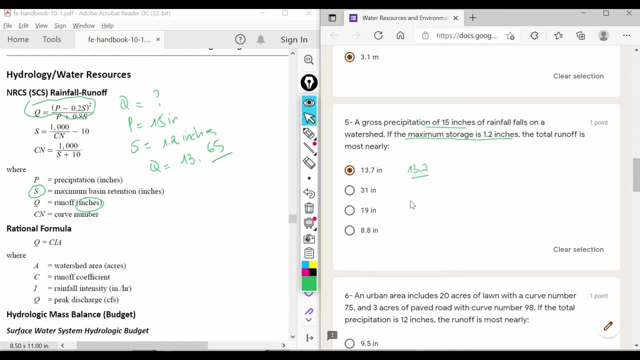 very close to 13.7 inches. so the good: very close to 13.7 inches. so the good answer here is this one. so let's move to answer. here is this one. so let's move to answer. here is this one. so let's move to the next question. so the next question. 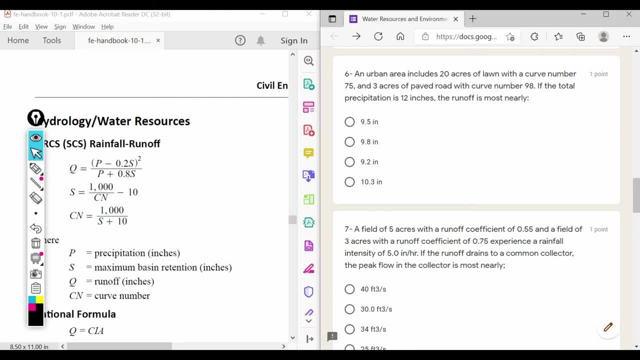 the next question, so the next question, the next question, so the next question is very similar to the previous one, but is very similar to the previous one. but is very similar to the previous one. but we have here two, two average. we have here two, two average. we have here two, two average, the curve number in order to find the 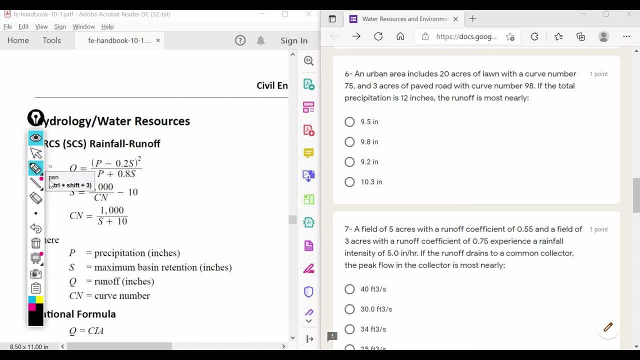 the curve number in order to find the, the curve number in order to find the solution. so what we have here, we have solution. so what we have here, we have solution. so what we have here we have: urban areas with first area is equal to. urban areas with first area is equal to. 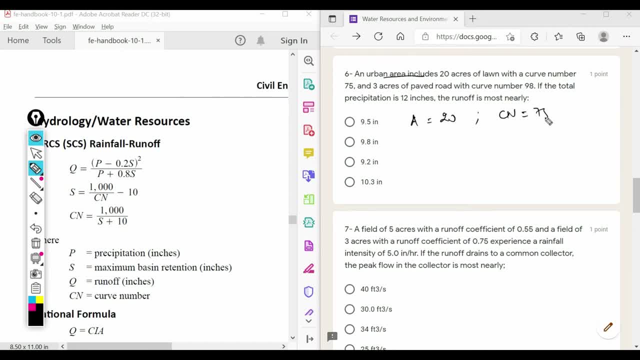 urban areas with: first area is equal to 20 acres with a curve number of 75 and 20 acres with a curve number of 75 and 20 acres with a curve number of 75, and second area has three acres with a curve. second area has three acres with a curve. 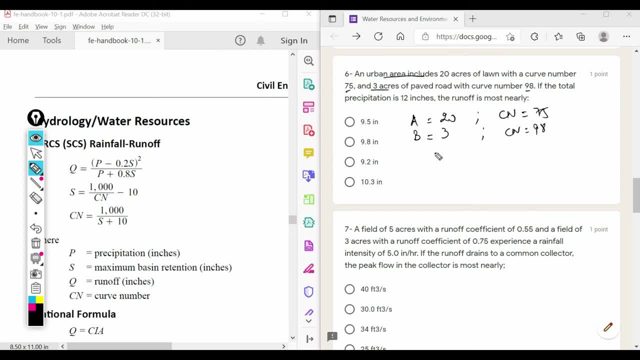 second area has three acres with a curve number with 98. so we use the same number with 98. so we use the same number with 98. so we use the same formula again, but we need to find first formula again, but we need to find first. 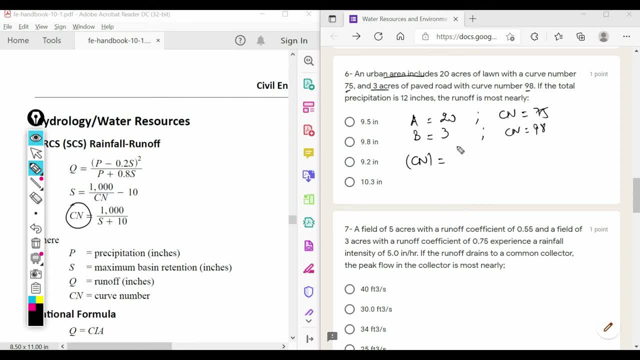 formula again. but we need to find first this CN, so the CN average, this CN, so the CN average, this CN, so the CN average is equal to area a multiply by its curve, is equal to area a multiply by its curve, is equal to area a multiply by its curve number, plus area B multiply by its curve. 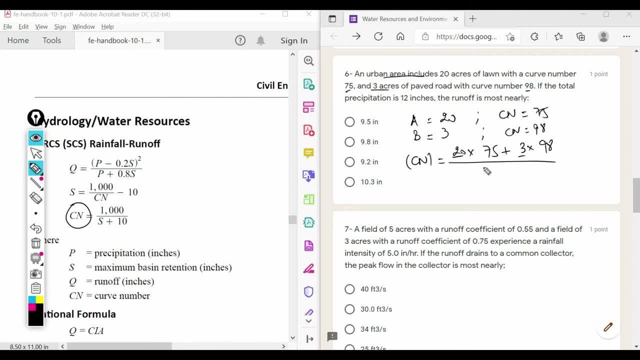 number plus area B multiply by its curve number plus area B multiply by its curve number over the sum of the areas 20 plus number, over the sum of the areas 20 plus number, over the sum of the areas 20 plus 3, so which gives us a value of of 78. so 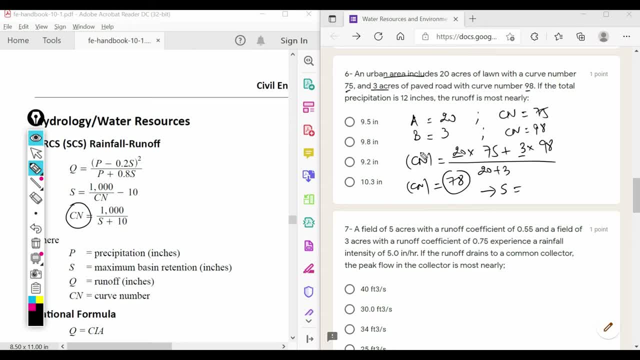 3 so, which gives us a value of of 78 so 3 so, which gives us a value of of 78, so, which means that s is equal to one, which means that s is equal to one, which means that s is equal to one thousands. so if we use this formula here, 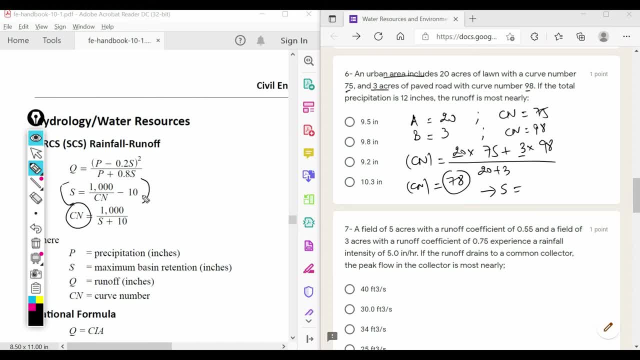 thousands. so if we use this formula here, thousands. so if we use this formula here, one thousands over 78 minus 10, which is one thousands over 78 minus 10, which is one thousands over 78 minus 10, which is equal to 2 points 8, 2. so finally, if we 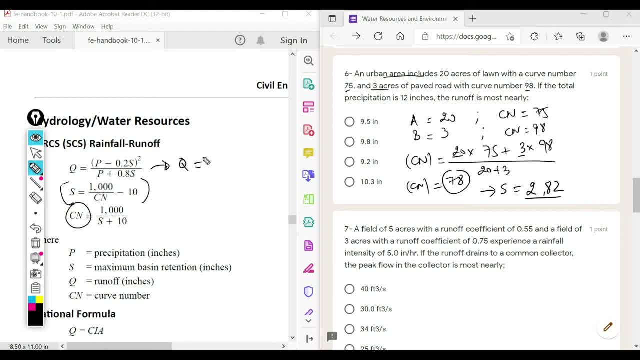 equal to 2 points 8, 2. so finally, if we equal to 2 points 8, 2. so finally, if we plug in the numbers here, we find that. plug in the numbers here, we find that. plug in the numbers here, we find that skewing inches is equal to. so here is. 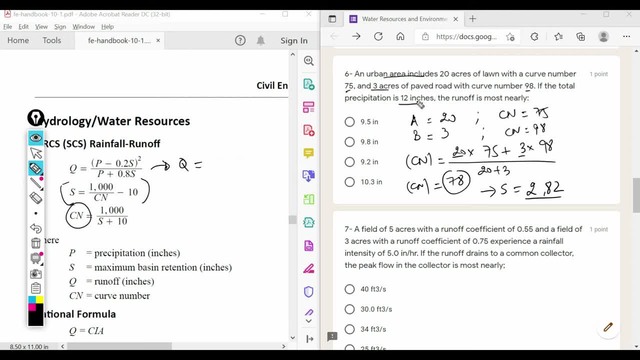 skewing inches is equal to so here is: skewing inches is equal to so. here is the P 12 inches minus 0.2 to this: the P 12 inches minus 0.2 to this: the P 12 inches minus 0.2 to this square over on 0.8. 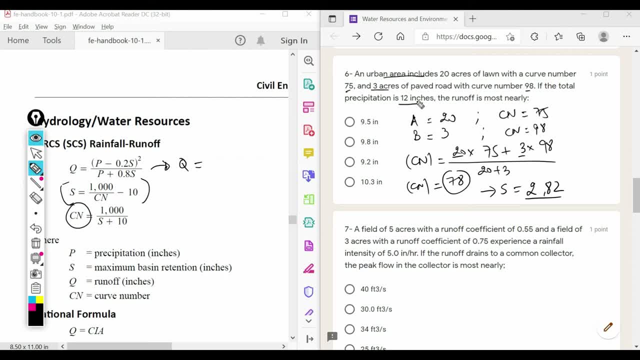 square over on 0.8. square over on 0.8. it's my way, this one here, so, and we'll it's my way, this one here so, and we'll it's my way, this one here so, and we'll find value of nine points. 17, which is: 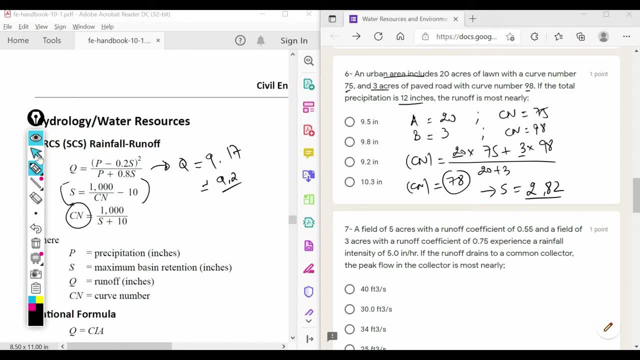 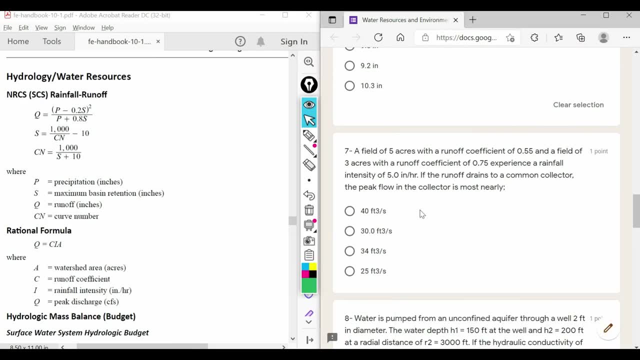 find value of nine points 17, which is find value of nine points 17, which is close to nine points two. so the good close to nine points two, so the good close to nine points two. so the good answer is C. so question number seven is: answer is C. so question number seven is: 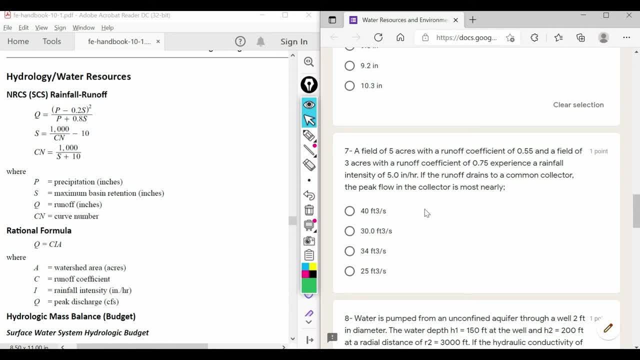 answer is C. so question number seven is about the other formula, which is the. about the other formula which is the, about the other formula, which is the rational formula. a field of five acres, rational formula. a field of five acres, rational formula. a field of five acres with the runoff coefficient, there is a 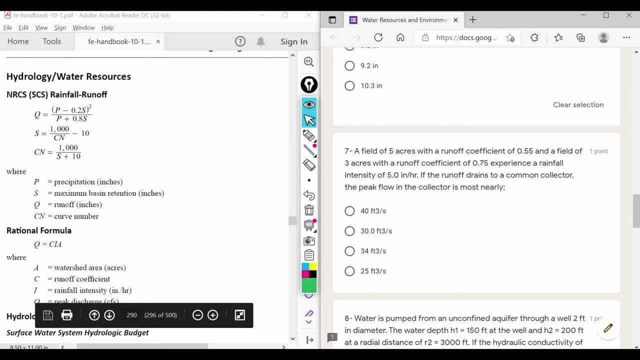 with the runoff coefficient, there is a. with the runoff coefficient, there is a runoff coefficient of zero. runoff coefficient of zero. runoff coefficient of zero: point fifty four, five and field of point fifty four, five and field of point fifty four, five and field of three acres. with the runoff coefficient of: 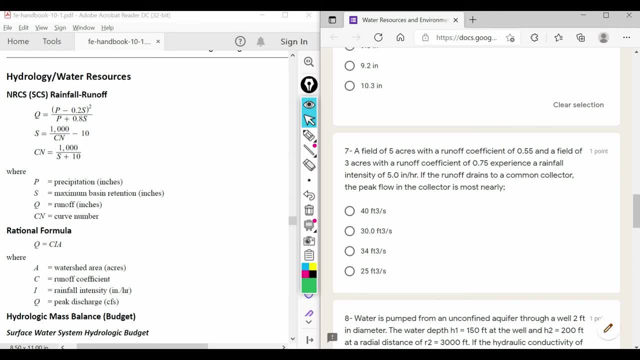 three acres with the runoff coefficient of three acres with the runoff coefficient of zero point seven. five experience a zero point seven. five experience a zero point seven. five experience a rainfall intensity of five inches per rainfall. intensity of five inches per rainfall. intensity of five inches per hour. if the runoff drains to a common. 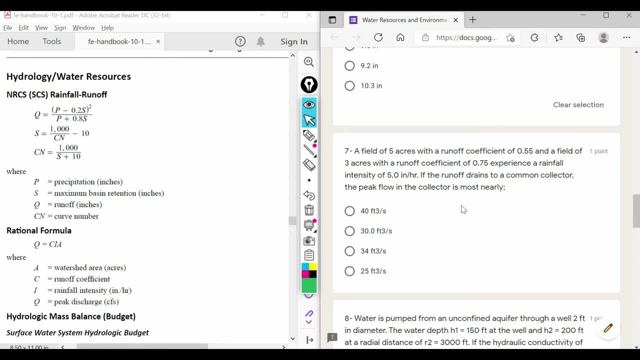 hour. if the runoff drains to a common hour. if the runoff drains to a common collector, the peak flow and the collector. the peak flow and the collector. the peak flow and the collector is most nearly. which of the collector is most nearly? which of the collector is most nearly which of the following? so the same goal calculating. 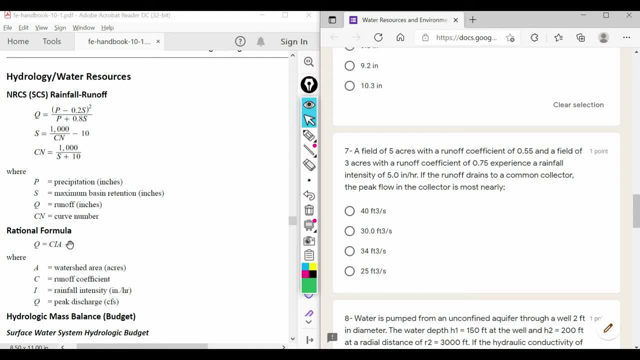 following, so the same goal: calculating. following. so the same goal: calculating the- the peak discharge, but with rational the the peak discharge, but with rational the the peak discharge, but with rational formula this time. so here we have in formula this time. so here we have in formula this time. so here we have. in order to calculate this formula, we need: 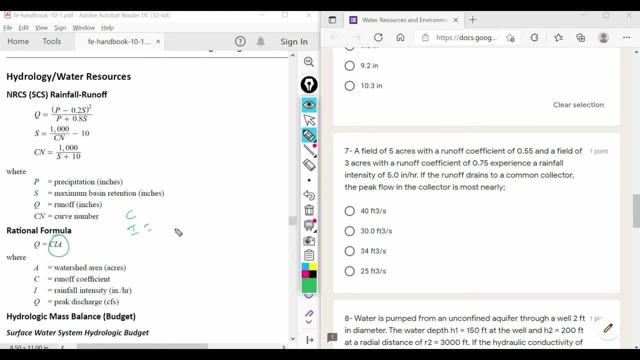 order to calculate this formula, we need order to calculate this formula- we need to calculate C I the rainfall intensity. to calculate C I the rainfall intensity. to calculate C I the rainfall intensity. which is given here somewhere, so here is. which is given here somewhere, so here is. 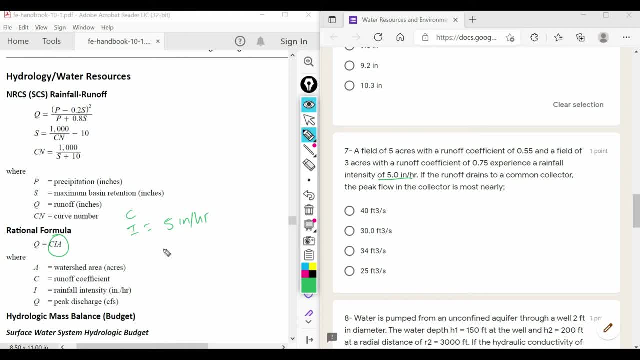 which is given here somewhere. so here is five inch per hour and we need to five inch per hour and we need to five inch per hour and we need to calculate the watershed area. watershed, calculate the watershed area. watershed, calculate the watershed area. watershed area is some of the area, so we have five. 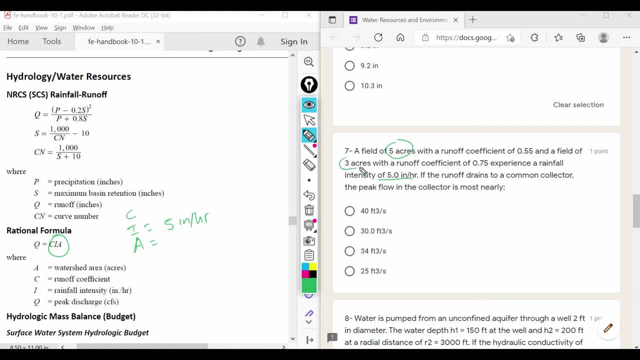 area is some of the area, so we have five area is some of the area, so we have five acres plus three acres, which is equal to acres, plus three acres, which is equal to acres, plus three acres, which is equal to eight acres. why we sum this areas? 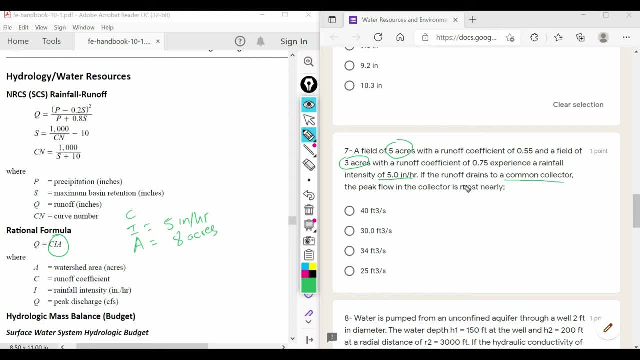 eight acres. why we sum this areas, eight acres. why we sum this areas? because we have a common collector for, because we have a common collector for, because we have a common collector for all these areas. so the runoff drains to all these areas. so the runoff drains to 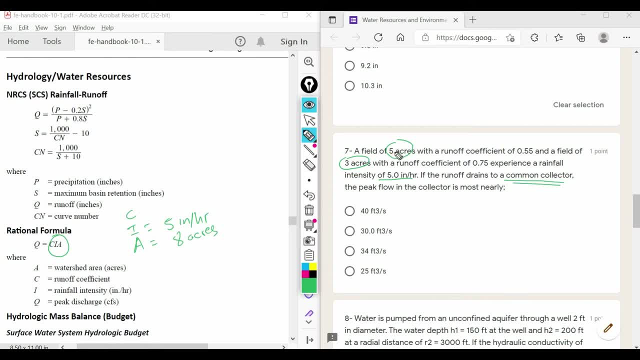 all these areas. so the runoff drains to a common collector, which means that this a common collector. which means that this a common collector, which means that this collector collects this area runoff plus collector collects this area. runoff plus collector collects this area. runoff plus this area. run and see. here will be. 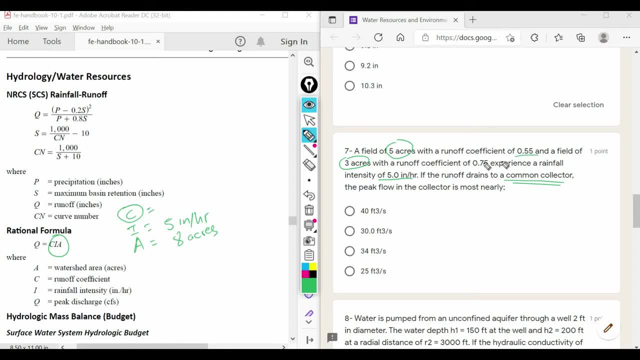 this area. run and see here will be this area. run and see here will be another C. because we have different another C. because we have different another C, because we have different values. we have 0.55 and 0.75, which means values. we have 0.55 and 0.75, which means 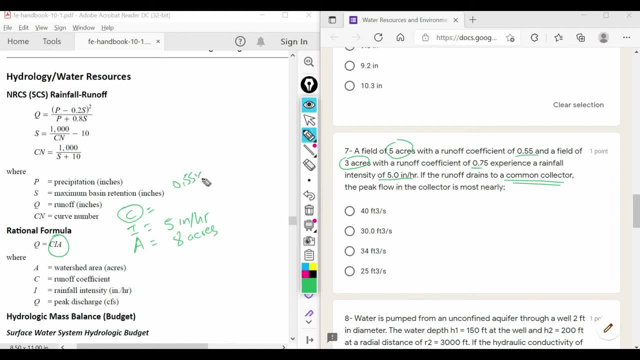 values. we have 0.55 and 0.75, which means that C will be an average x, the that C will be an average x, the that C will be an average x. the first surface, which is equal to 5 plus the first surface, which is equal to 5 plus the. 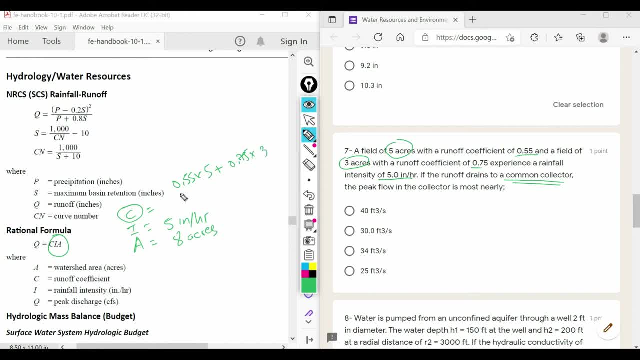 first surface which is equal to 5 plus the second. one x second surface over the second. one x second surface over the second. one x second surface over the sum of the surfaces or the areas which sum of the surfaces, or the areas which sum of the surfaces or the areas, which means that C will be equal to 3 over 8. 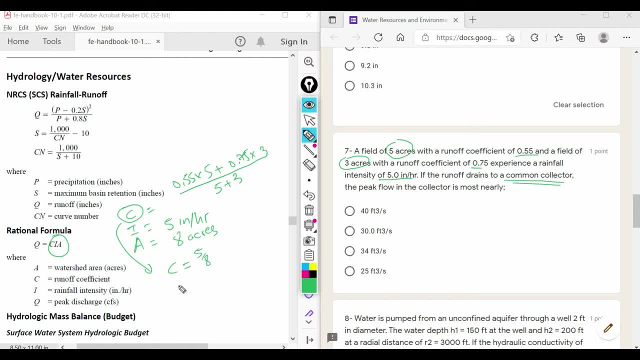 means that C will be equal to 3 over 8. means that C will be equal to 3 over 8, so 5 over 8, so 5 over 8, so 5 over 8. so now let's do the math. Q will be equal to. 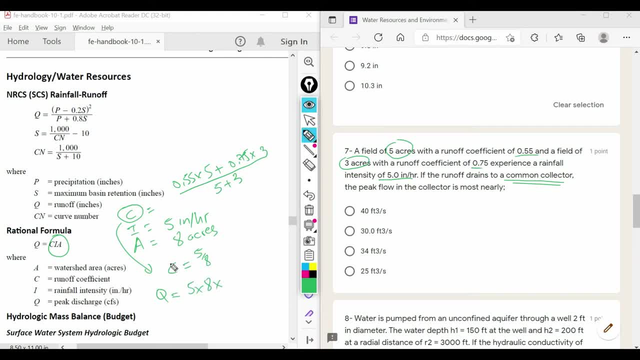 so now let's do the math. Q will be equal to. so now let's do the math. Q will be equal to 5 x 8 x C, which is 5 over 8. so Q is 5 x 8 x C, which is 5 over 8. so Q is: 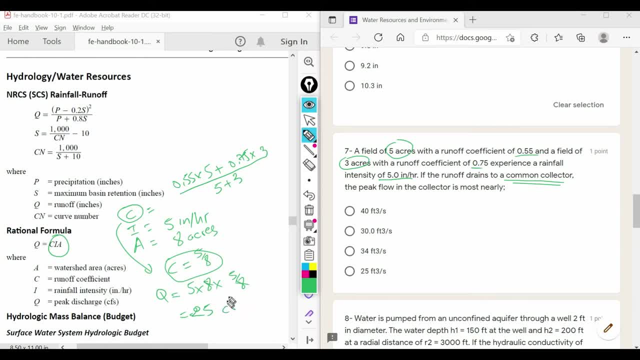 5 x 8 x C, which is 5 over 8. so Q is equal to 25 cubic foot per second. so the equal to 25 cubic foot per second. so the equal to 25 cubic foot per second. so the good answer here, or the exact answer, is: 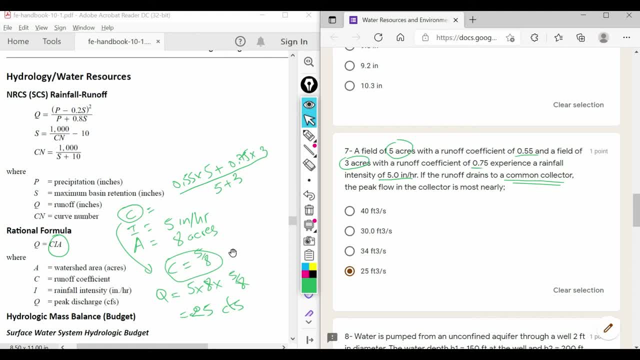 good answer here, or the exact answer is good answer here, or the exact answer is this one, and here we have to notice this one, and here we have to notice this one, and here we have to notice something very interesting, this formula, something very interesting, this formula, something very interesting. this formula works, whether you have 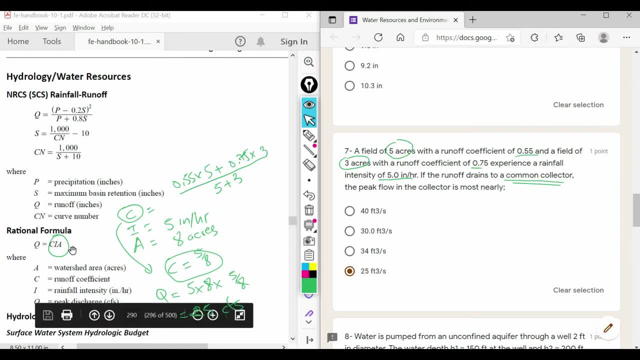 works, whether you have works, whether you have this units or the international system, this units or the international system, this units or the international system of units. you can use the same formula of units. you can use the same formula of units. you can use the same formula having the international system of units. 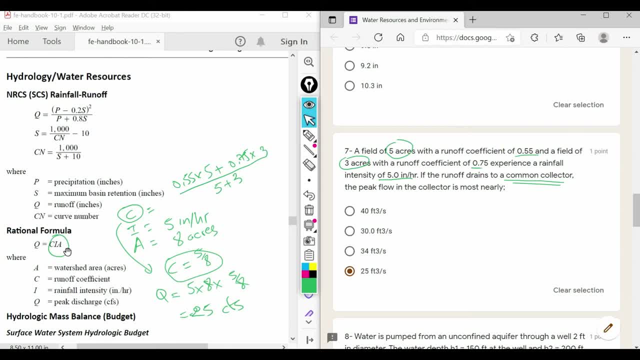 having the international system of units, having the international system of units because it's a homogeneous equation, the because it's a homogeneous equation, the because it's a homogeneous equation. the units of C multiplied by E, multiplied by units of C multiplied by E, multiplied by units of C multiplied by E multiplied by a, will give you the units of Q which 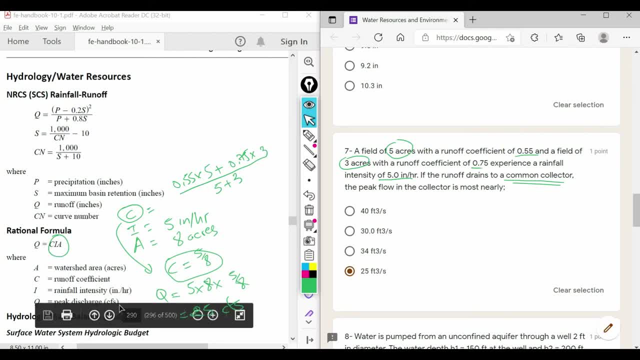 a will give you the units of Q, which a will give you the units of Q, which means that you can either use the means that you can either use the means that you can either use the international system or this units here: international system or this units here. 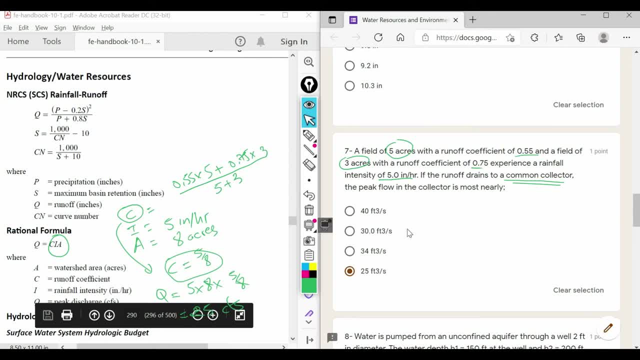 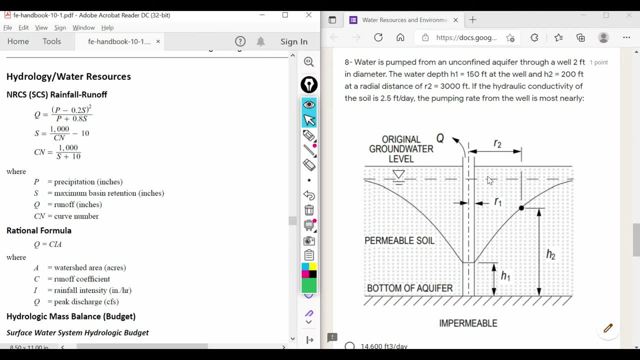 international system or this units here to find the results. so let's move to the to find the results. so let's move to the to find the results. so let's move to the next question. so question number eight. next question. so question number eight. next question, so question number eight. it's about: well, original, okay water is. 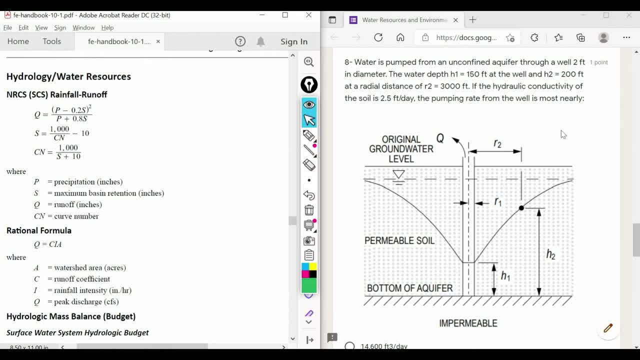 it's about well original, okay water is. it's about well, original, okay water is pumped from an unconfined aquifer. pumped from an unconfined aquifer. pumped from an unconfined aquifer through well of two feet in diameter, the through well of two feet in diameter, the. 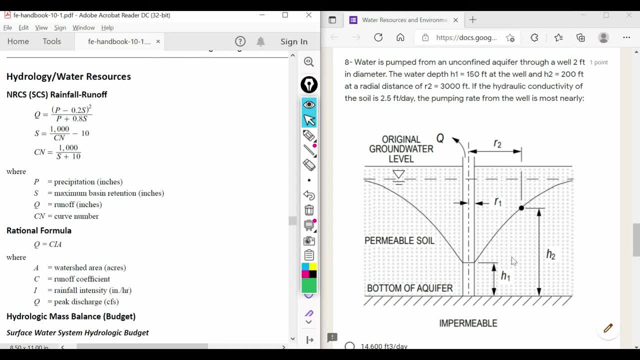 through well of two feet in diameter. the water depth: h1 is equal to this at the water depth. h1 is equal to this at the water depth. h1 is equal to this at the well and h2 is equal to 200 feet at well and h2 is equal to 200 feet at. 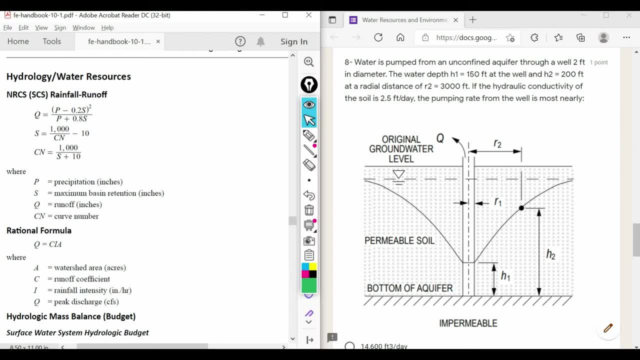 well, and h2 is equal to 200 feet at radial distance. r2 equal to 3000 feet. in radial distance. r2 equal to 3000 feet in radial distance. r2 equal to 3000 feet. in the hydraulic if the hydraulic, the hydraulic if the hydraulic. 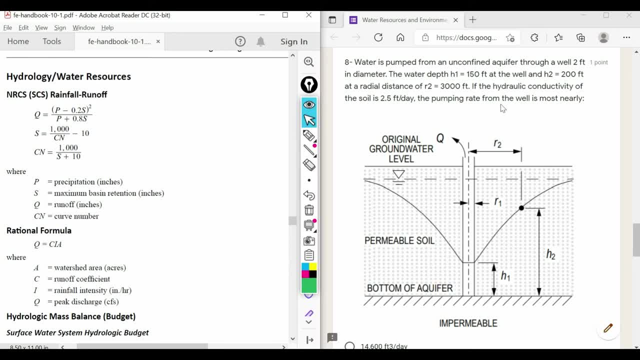 the hydraulic. if the hydraulic conductivity on soil is 2.5 feet per day, conductivity on soil is 2.5 feet per day. conductivity on soil is 2.5 feet per day. the pumping rate from the well is most. the pumping rate from the well is most. 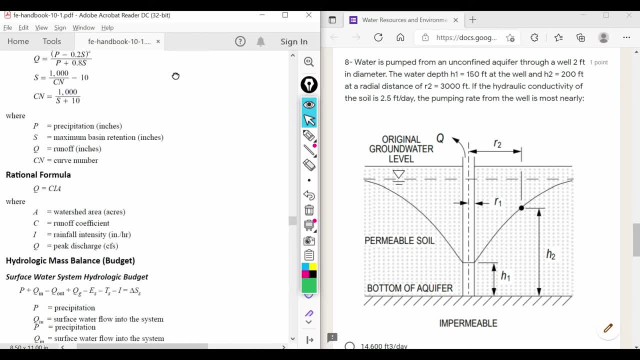 the pumping rate from the well is most nearly which of the following. so here we nearly. which of the following. so here we nearly which of the following. so here we. knew we need to use the well formula. knew we need to use the well formula. knew we need to use the well formula here. after Darcy, low, yeah, we have the. 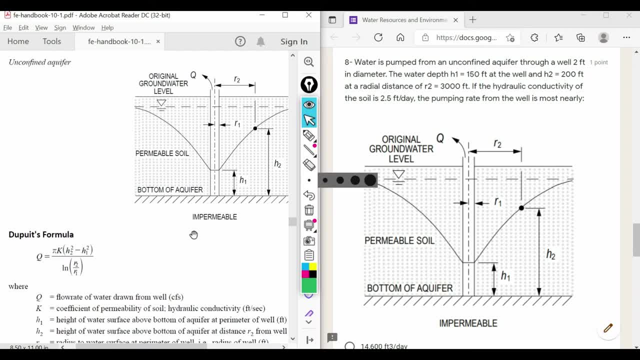 here after Darcy: low yeah, we have the here after Darcy- low yeah, we have the well draw down. so we have unconfined well draw down. so we have unconfined well draw down. so we have unconfined aquifer, which is our case here, and we 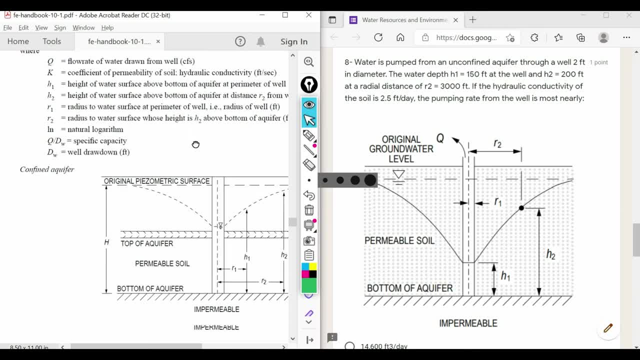 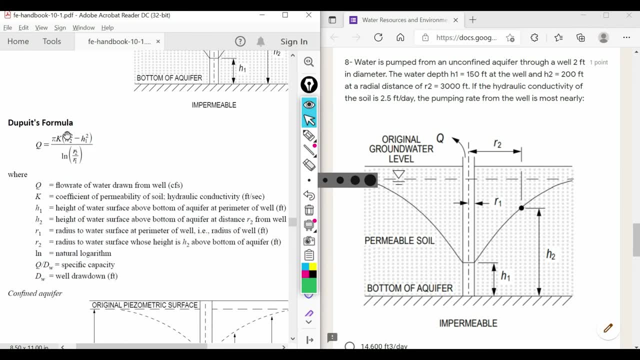 aquifer, which is our case here, and we aquifer, which is our case here, and we have a confined aquifer. so here we'll have a confined aquifer. so here we'll have a confined aquifer. so here we'll use the, the first formula, the pre's. 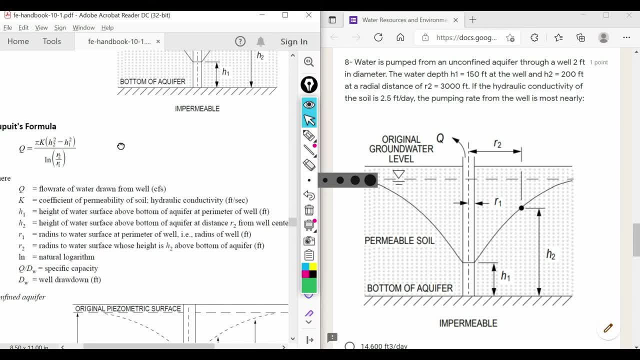 use the, the first formula, the pre's. use the, the first formula, the pre's. formula about that: we find aquifer. so formula about that: we find aquifer. so formula about that: we find aquifer. so let's figure out the things we need here. let's figure out the things we need here. 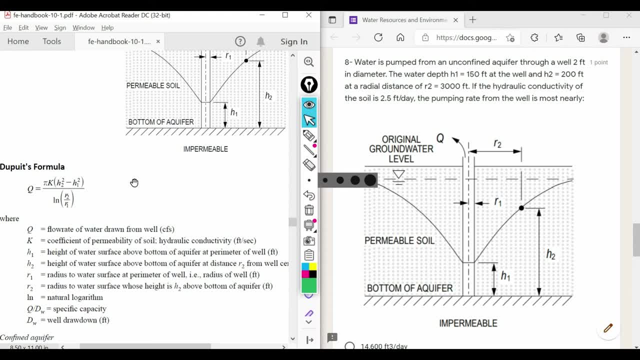 let's figure out the things we need here in order to solve the problem. so what we in order to solve the problem, so what we in order to solve the problem. so what we are looking for, we are looking for are, are looking for, we are looking for are. 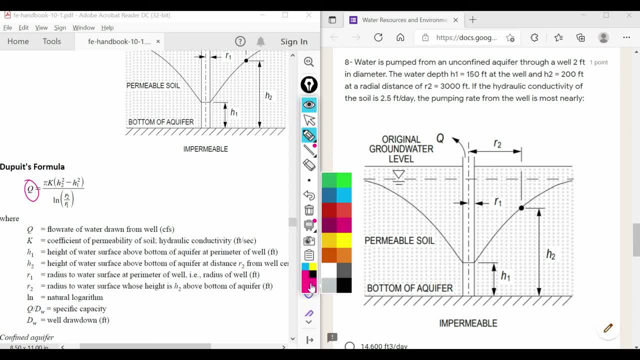 are looking for, we are looking for, are looking for you. this is our and now looking for you. this is our and now looking for you. this is our and now, and what we know so far. we know the the K and what we know so far. we know the the K. 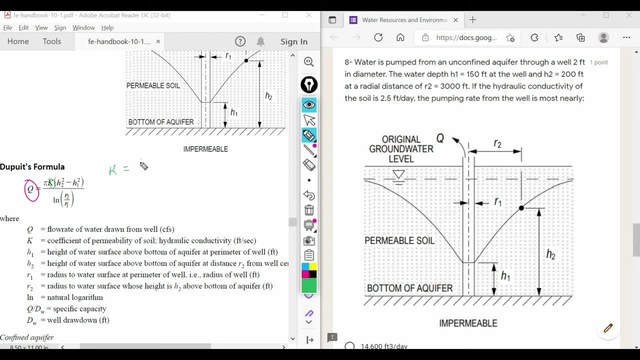 and what we know so far. we know the, the K, so K is equal to 2.5 feet per day, so K is equal to 2.5 feet per day, so K is equal to 2.5 feet per day. notice, that's you. this has to be. 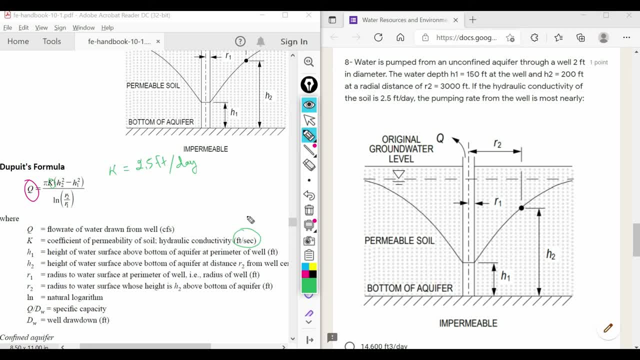 notice, that's you. this has to be. notice, that's you. this has to be expressed in foot per seconds, but wait. a. expressed in foot per seconds, but wait. a expressed in foot per seconds, but wait a minute. the question is asking about the minute. the question is asking about the. 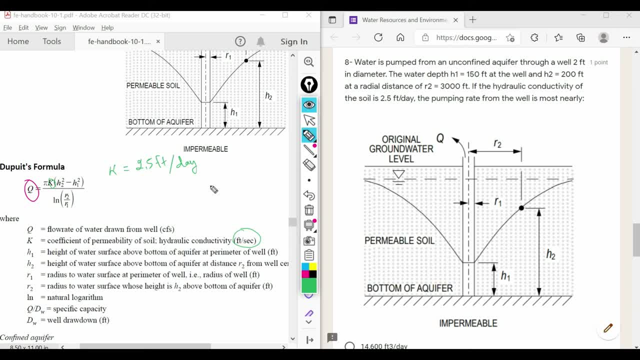 minute. the question is asking about the pumping rate in foot, cubic foot per day. pumping rate in foot, cubic foot per day. pumping rate in foot, cubic foot per day. so we don't need to transform it to so we don't need to transform it to. so we don't need to transform it to seconds and then transform it back today. 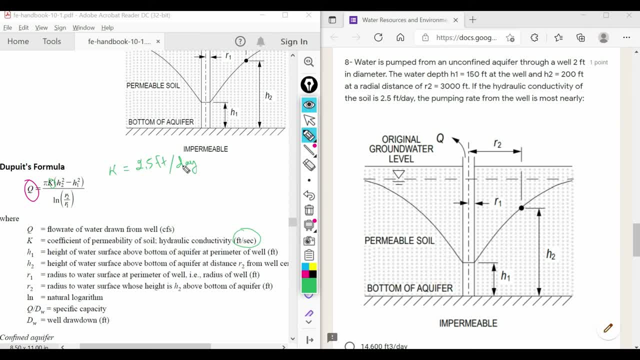 seconds and then transform it back today seconds and then transform it back today, so we'll lose time. so let's just keep it. so we'll lose time. so let's just keep it. so we'll lose time. so let's just keep it here in days, because we want the results. 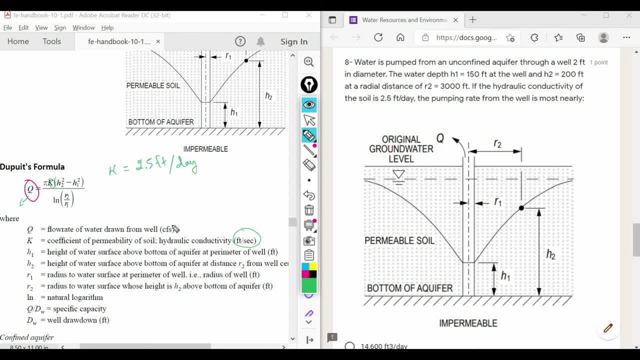 here in days because we want the results here in days, because we want the results here in cubic foot per day and not cubic here in cubic foot per day and not cubic here in cubic foot per day and not cubic foot per second in this exercise. so h2. 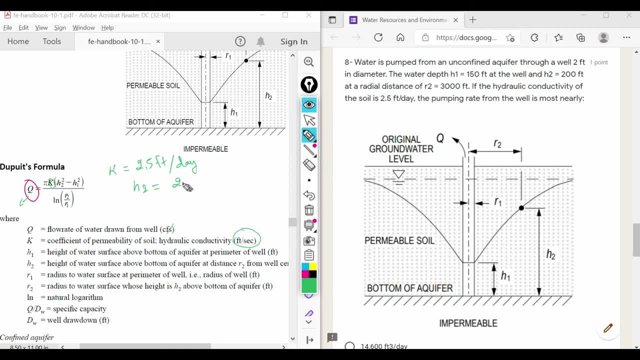 foot per second in this exercise. so h2 foot per second in this exercise. so h2 is equal to 200 feet, which is the good is equal to 200 feet, which is the good is equal to 200 feet, which is the good units. h1 is equal to one hundred fifty. 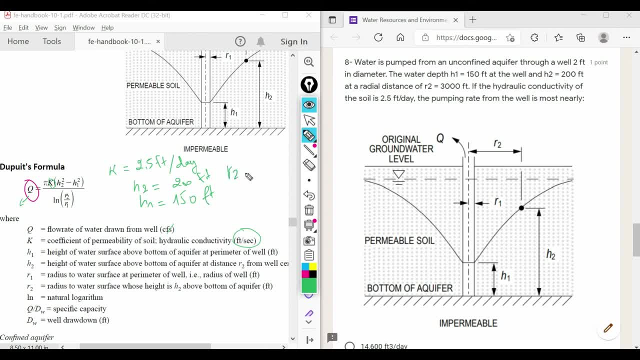 units. h1 is equal to one hundred fifty units. h1 is equal to one hundred fifty feet. r2 is equal to three thousand feet feet. r2 is equal to three thousand feet feet, r2 is equal to three thousand feet and r1. this is the tricky one. the tricky. 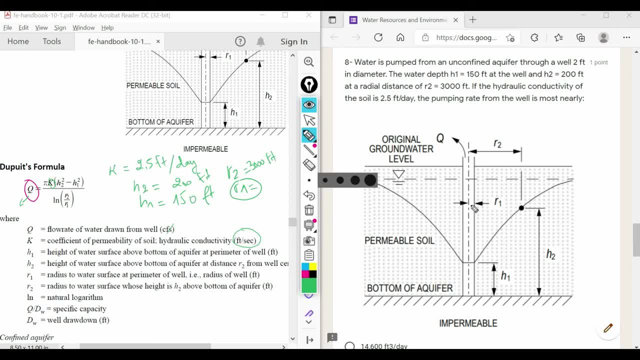 and r1- this is the tricky one, the tricky. and r1- this is the tricky one, the tricky one. r1 is not equal to 2. r1 is equal to one. r1 is not equal to 2. r1 is equal to one. r1 is not equal to 2. r1 is equal to 2 over 2, so it's not diameter, but it's a. 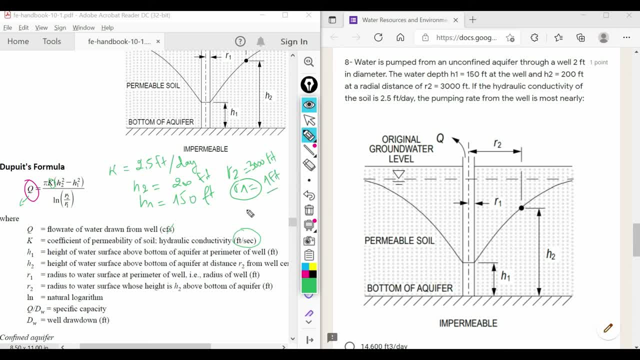 2 over 2, so it's not diameter, but it's a 2 over 2, so it's not diameter, but it's a radius. so here is the tricky one, and if radius? so here is the tricky one, and if radius. so here is the tricky one, and if you choose, here two feet. 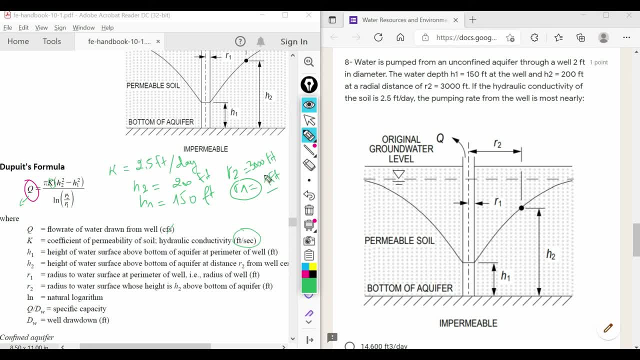 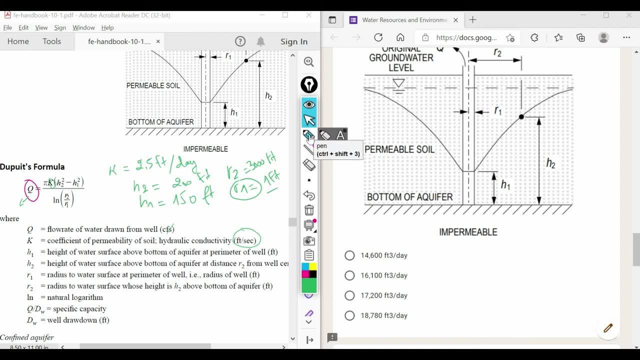 you choose here two feet instead of one feet, you will find the wrong answer, which is here. I think you will find this answer here and let's just plug in the numbers right now. so we have Q equal P, P multiplied by 2.5, multiplied by h2 square minus h1 square. 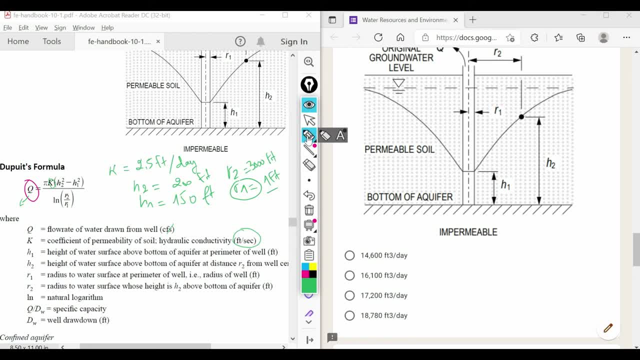 over ln of r2 over 1, which is equal to approximately seventy thousand one six six point nine two, but which is closest to this value here. so the closest answer here is this one. so let's move to the next question. so question is: what is the answer to this question? so the answer to this question is: 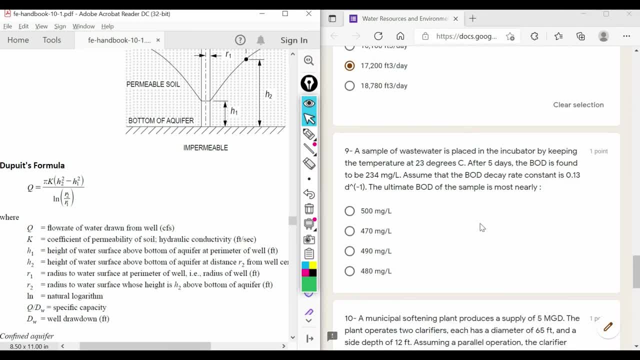 number nine is about the whole decay rates. so sample of wastewater is placed in an incubator by keeping the temperature at 23 degrees. after five days the board is found to be two, three, four milligram per liter. assume that the body K rate consent is 0.3 day to the minus one power or over day, the ultimate. 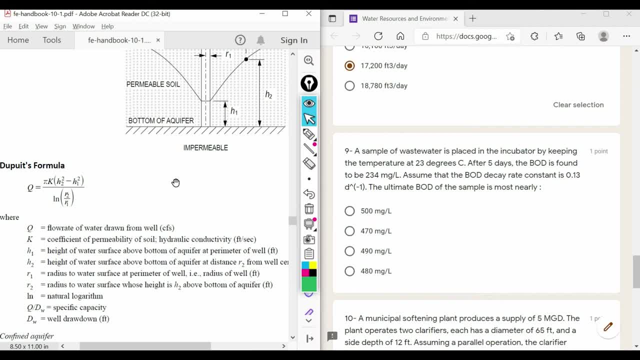 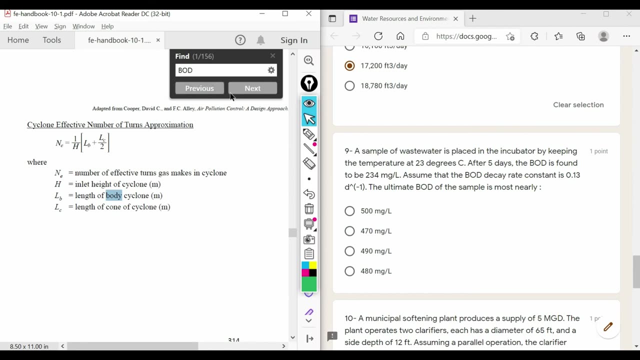 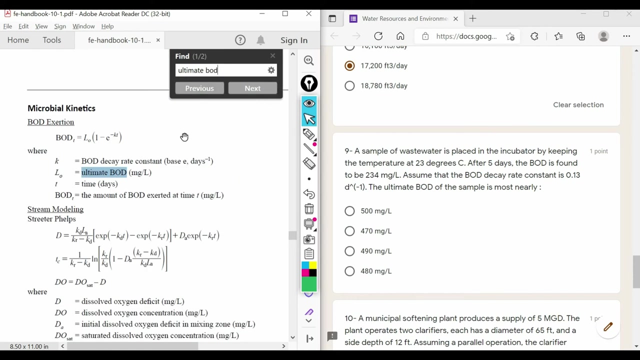 both of the sample is most nearly so. here we have to find the formula that links the bold, the ultimate world or the infinite void to the precise void or void after certain period of time. so let's use here both. okay, so we have to use it to find it quickly. use a team. 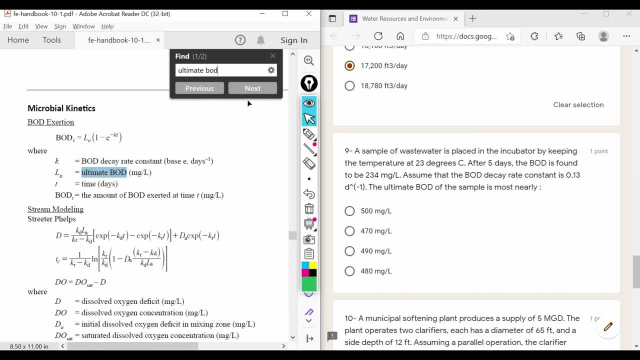 it's bold and you will find it very quickly. so this is the formula here and that we have to use in order to solve this problem. so this is our formula and what we have. we have bold T. T is expressed in days. it's equal here to: 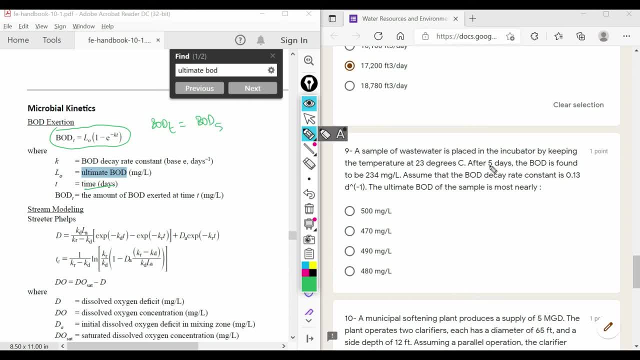 boy, both five. so we have the world out after five days. so this value is expressed in the units that we have to use here, so we don't have to care about units. so two, three, four milligrams, uh per liter. so this one is okay. now we need l zero. l zero is 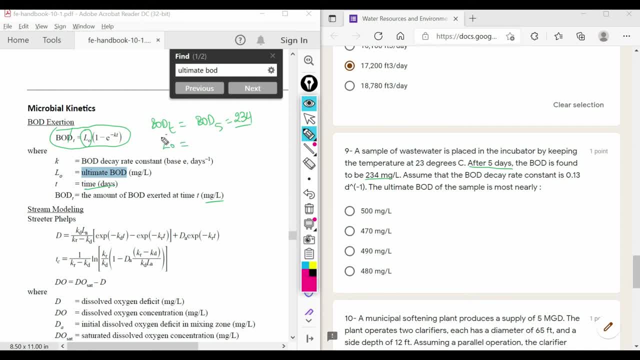 what we are looking for. it's our anon, so in zero, we keep it. so it's our anon. and now let's move to this here: minus kt, t, so minus k. minus k is the decay rate constant, which is equal here to 0.13, and t is the time in days, so t in our case it's five days, okay, so uh, let's use uh again. 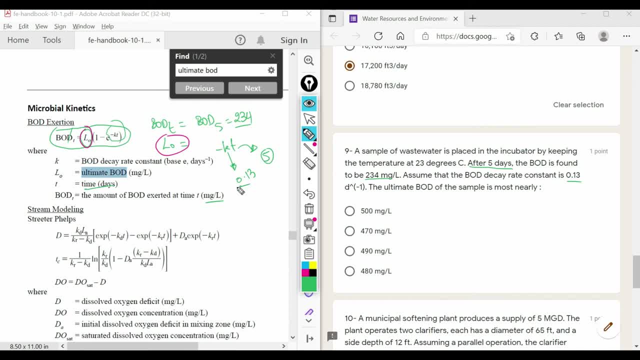 uh, uh. so you have to just plug and chug and you will find the formula. so you'll find the so l zero here is equal to the both at five days, which is equal to two, three, four over one minus uh exponent to minus uh k, which is equal to 0.13 multiplied by five, and the good answer is one minus uh. 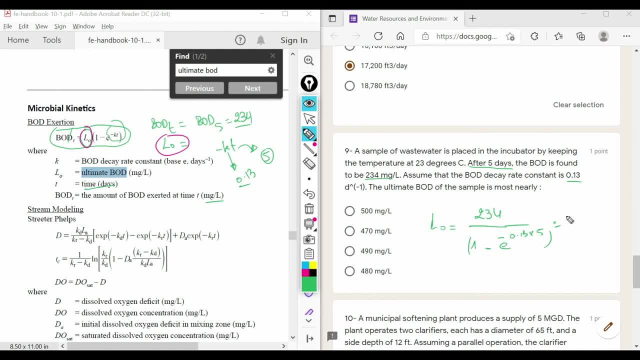 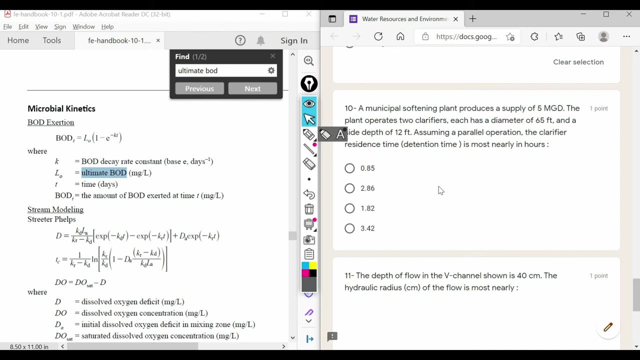 minus 0.13 multiplied by five, so it's equal. l zero is equal to four, eight nine point six, which is close to this value here. so the good answer is c. let's move to next question. so for, uh, this question, question number 10. um, i think it's an easy question. the difficult thing about this question: 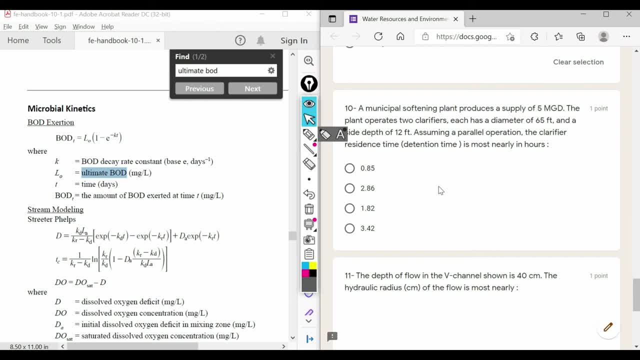 is the unit that you have to convert before to find the results in our. but to give you a quick idea about about what we are looking for, let's just do a dimensional analysis here. let's forget about what we know about clarifiers, produce, supply, etc. so here we have the first, the first quantity. 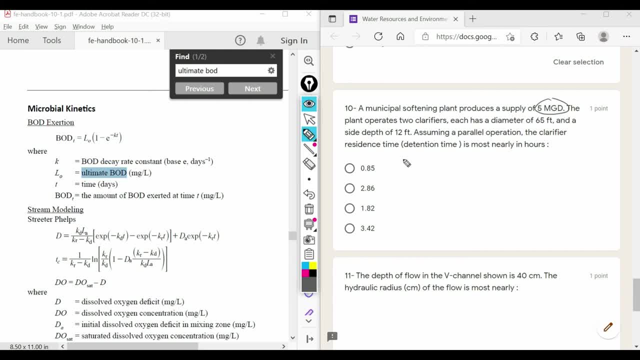 is expressed as mega million is expressed as mega million. gallons per day, which is a volume. gallons per day, which is a volume. gallons per day, which is a volume per time, and in the other side we have per time, and in the other side we have per time and in the other side we have uh, dimensions of the clarifiers. 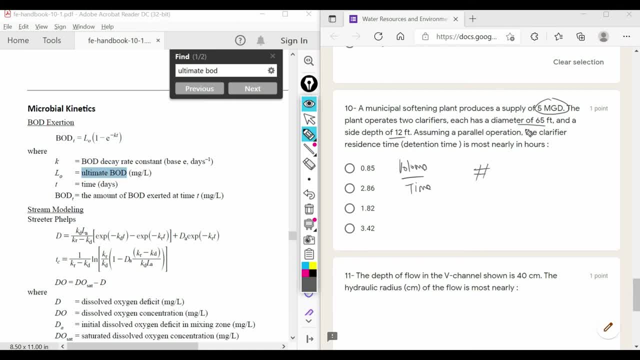 uh dimensions of the clarifiers. uh dimensions of the clarifiers, diameter and depth, and the diameter will diameter and depth, and the diameter will diameter and depth, and the diameter will gives us the section and the depth will gives us the section and the depth will gives us the section and the depth will gives us the volume. so this one and this, 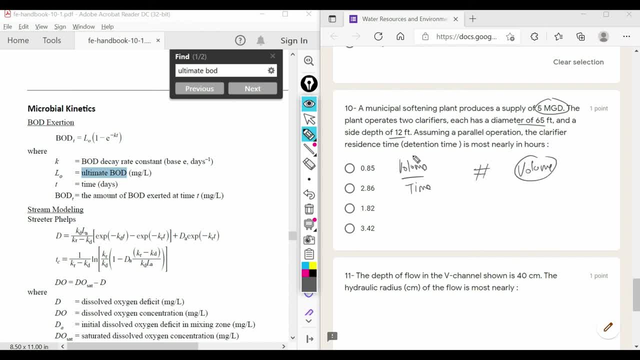 gives us the volume. so this one and this gives us the volume. so this one and this one will gives us the volume, one will gives us the volume, one will gives us the volume. so what we need to find the time we need. so what we need to find the time we need. 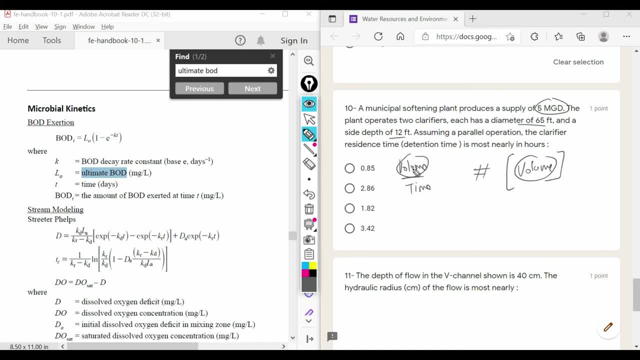 so what we need? to find the time, we need to divide this one, this quantity here, to divide this one, this quantity here, to divide this one, this quantity here, by this quantity here, because volume by this quantity here, because volume by this quantity here, because volume over over. 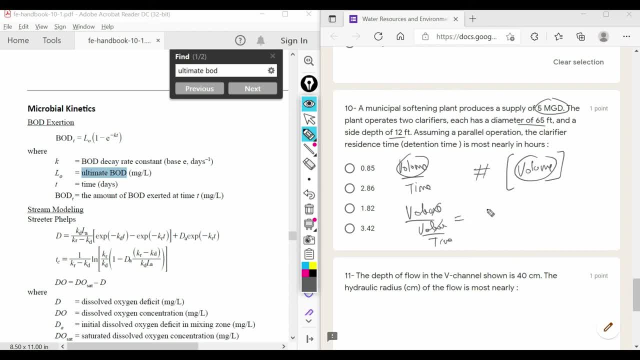 over volume over time. volume over time. volume over time is equal to time, is equal to time, is equal to time. so what we are looking for is a time. so what we are looking for is a time. so what we are looking for is a time. so now let's uh. 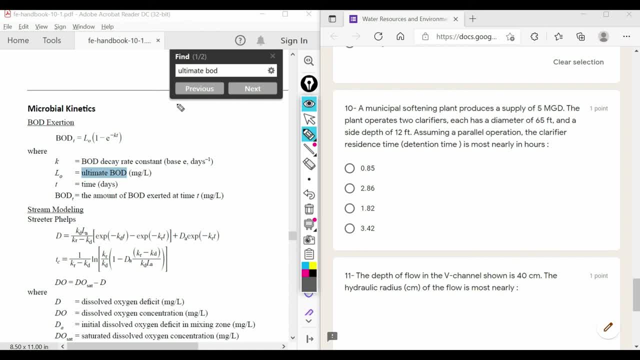 so now let's uh, so now let's uh, express the logic behind. so. the supply express the logic behind so the supply express the logic behind. so the supply. daily supply is daily. supply is daily. supply is five million gallon per day, but in order. five million gallon per day, but in order. 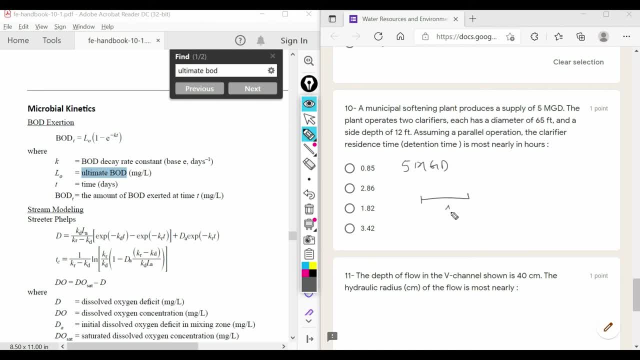 five million gallon per day. but in order to do this, to do this, to do this, we have two qualifiers qualifier number. we have two qualifiers qualifier number. we have two qualifiers: qualifier number one, one one and qualifier number two, which are: and qualifier number two, which are, and qualifier number two, which are identical. 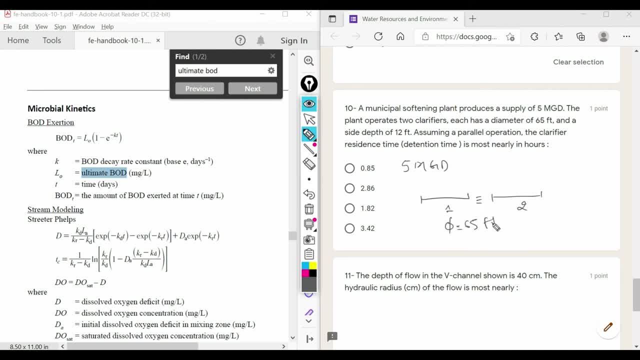 identical. identical, so the they have a diameter of 65 feet, so the they have a diameter of 65 feet, so the they have a diameter of 65 feet and a depth of 12 feet. so what are the? and a depth of 12 feet. so what are the? 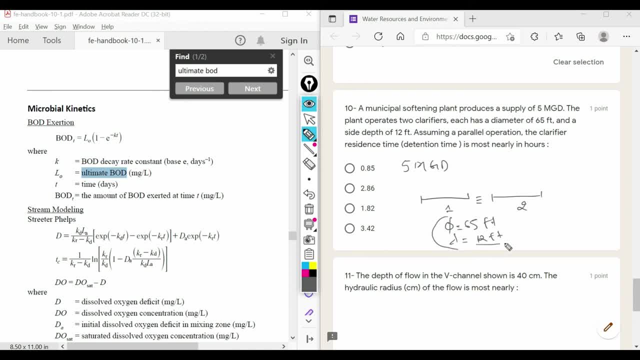 and a depth of 12 feet. so what are the volumes that are produced? volumes that are produced, volumes that are produced, that can be produced by these two, that can be produced by these two, that can be produced by these two qualifiers: is the volume of one of them. 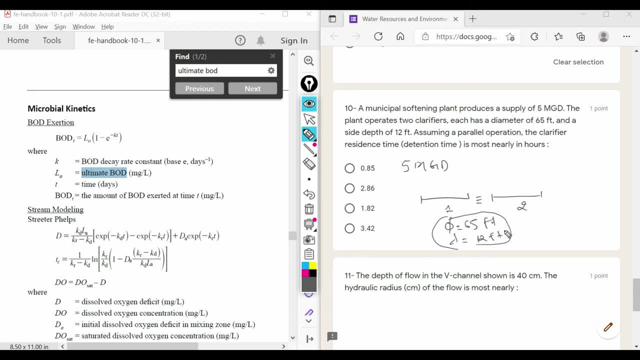 qualifiers is the volume of one of them. qualifiers is the volume of one of them multiplied by two, multiplied by two, multiplied by two. so if we multiply that by by the time, so if we multiply that by by the time, so if we multiply that by by the time we will have by number of hours per day. 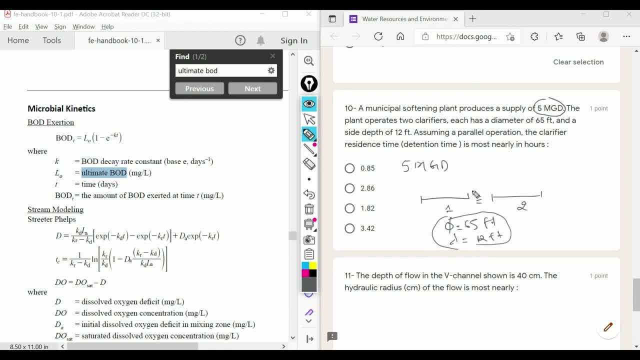 we will have by number of hours per day. we will have by number of hours per day. we'll have this, we'll have this, we'll have this value here. so that's why the value here. so that's why the value here, so that's why the answer will be equal to: 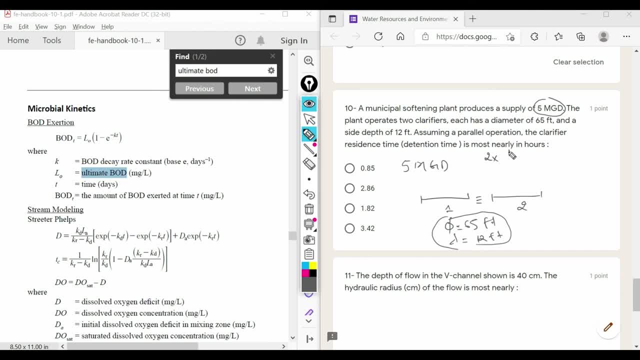 answer will be equal to answer will be equal to 2 multiplied by the volume, which is 2 multiplied by the volume, which is 2 multiplied by the volume, which is equal to, equal to, equal to p over 4 multiplied by 65. to find the. 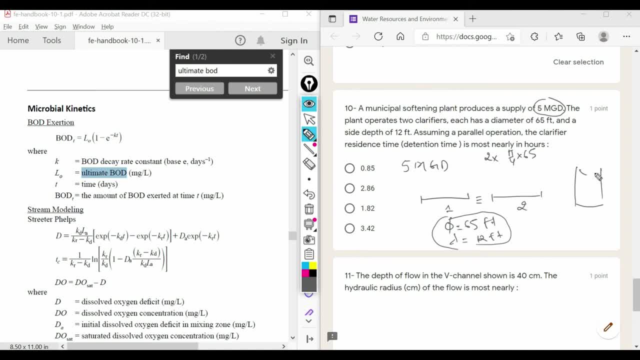 p over 4 multiplied by 65. to find the p over 4 multiplied by 65. to find the section. because section, because section, because qualifier is like cylinders, so and the qualifier is like cylinders so and the qualifier is like cylinders so and the volume of cylinder is the area of the 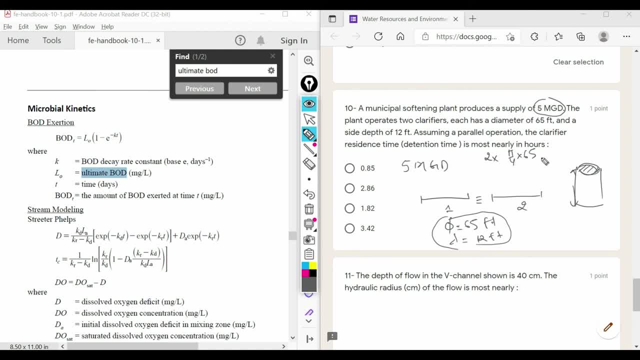 volume of cylinder is the area of the volume of cylinder, is the area of the circle multiplied by the depth. the area circle multiplied by the depth. the area circle multiplied by the depth. the area of the circle is this one and the depth of the circle is this one and the depth. 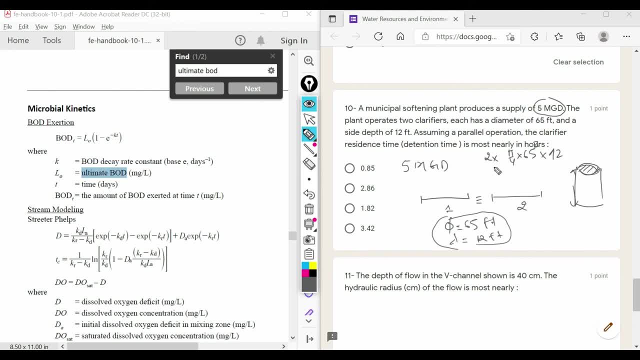 of the circle is this one, and the depth is is: is uh 12, uh 12, uh 12, okay, okay, okay. and now we have to divide this, but don't. and now we have to divide this, but don't. and now we have to divide this, but don't forget that this one is expressed in 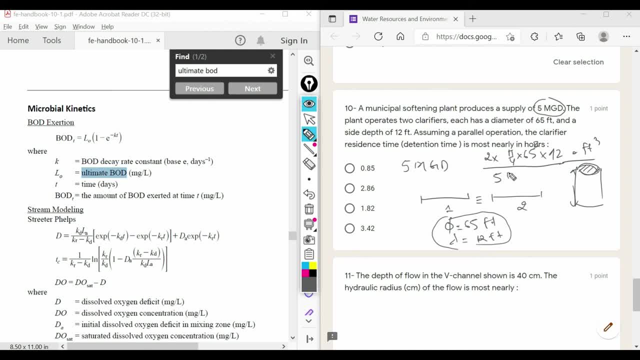 forget that this one is expressed in. forget that this one is expressed in feet, feet, feet. you have to divide this by five. you have to divide this by five. you have to divide this by five million gallon, million, gallon, million gallon per day, per day. so we need to transform. 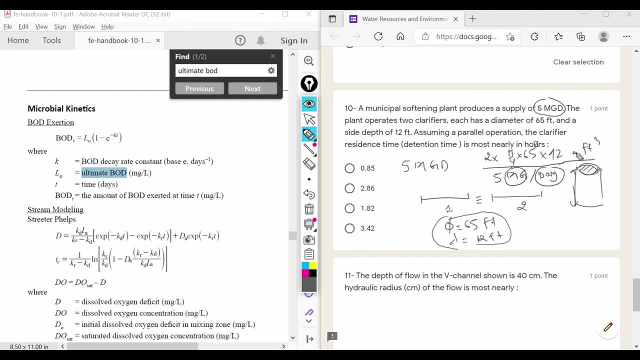 so we need to transform. so we need to transform million gallons, million gallons, million gallons to feet, to feet, to feet. uh to feed cube, uh to feed cube, uh to feed cube. and days to hours in order to find final, and days to hours in order to find final. 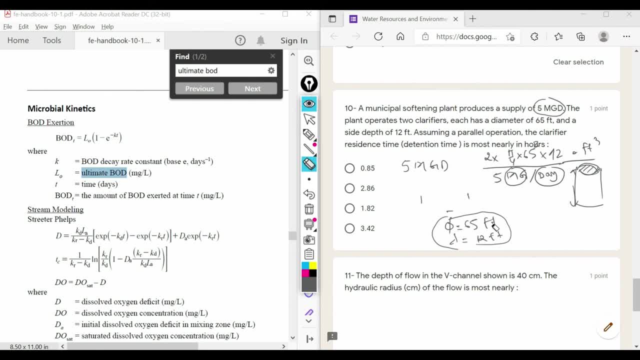 and days to hours in order to find final answer. answer, answer, so let's, uh, let's do it so if you um, if you have to, let's do it. so if you um, if you have to, let's do it so if you um, if you have to, you forget, for example, gallons to fruit. 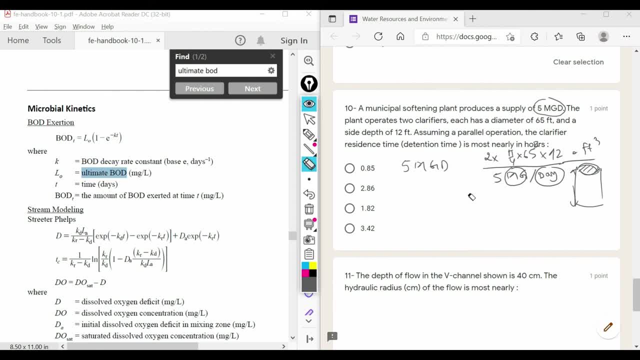 you forget, for example, gallons to fruit. you forget, for example, gallons to fruit. and if you don't use your calculator in and if you don't use your calculator in and if you don't use your calculator, in my case, my calculator gives me. my calculator gives me. 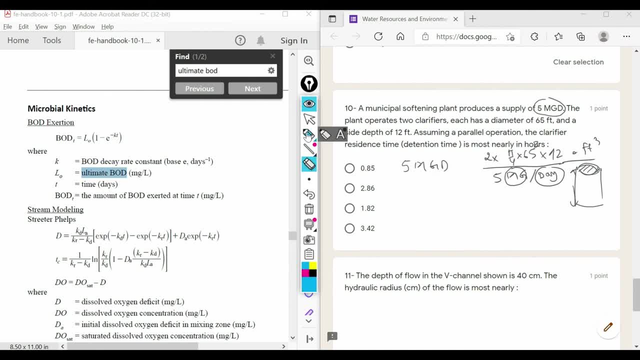 my calculator gives me um gallons. give me gallons to um gallons. give me gallons to um gallons. give me gallons to uh liters, uh liters, uh liters. and since i, i know that one meter is, and since i, i know that one meter is, and since i, i know that one meter is equal to, 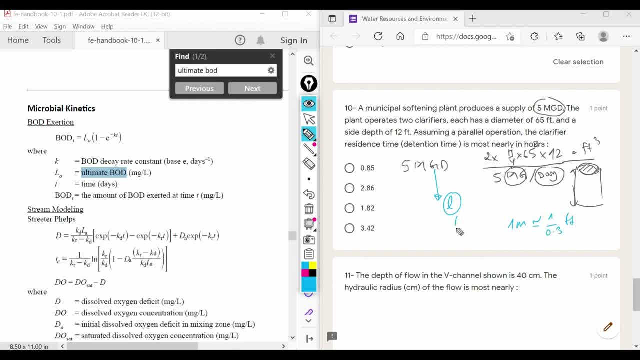 equal to equal to uh 1 over 0.3 foot. i can transform this: uh 1 over 0.3 foot. i can transform this: uh 1 over 0.3 foot. i can transform this to meter cube and then to foot cube, but to meter cube and then to foot cube, but to meter cube and then to foot cube. but you don't have to use this. you can find you don't have to use this. you can find you don't have to use this. you can find this in your. 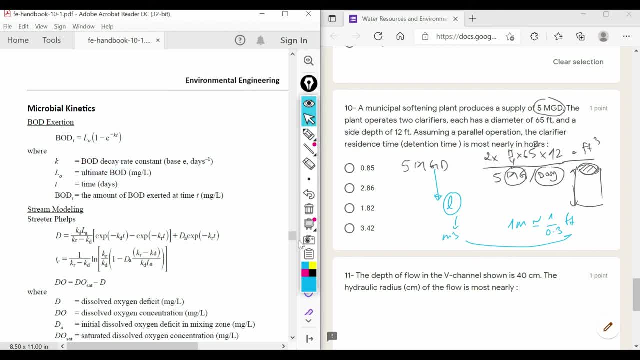 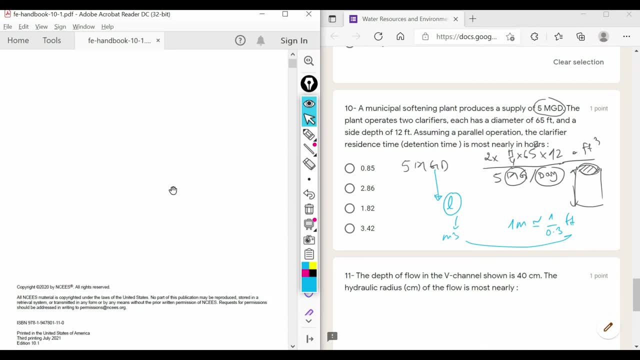 this in your, this in your in your handbook. so let's move to the to in your handbook. so let's move to the to in your handbook. so let's move to the to the first pages. uh, so here we can find quickly the units we are. we can find quickly the units we are. 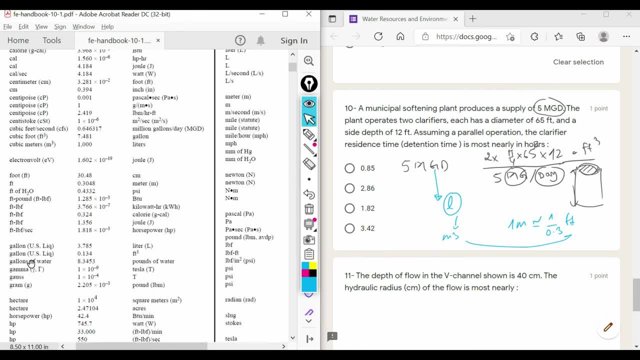 we can find quickly the units we are looking for. so here we have gallon and here we have. so here we have gallon and here we have. so here we have gallon and here we have foot square. so we know that from this foot square, so we know that from this. 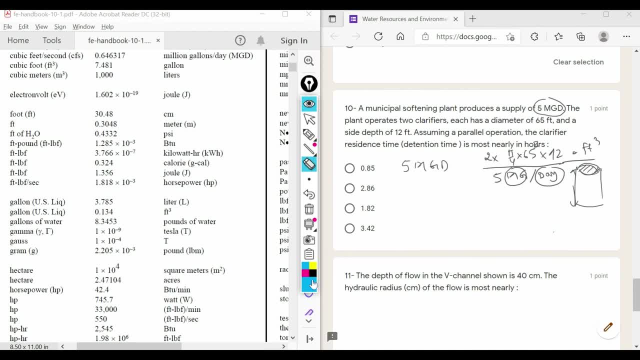 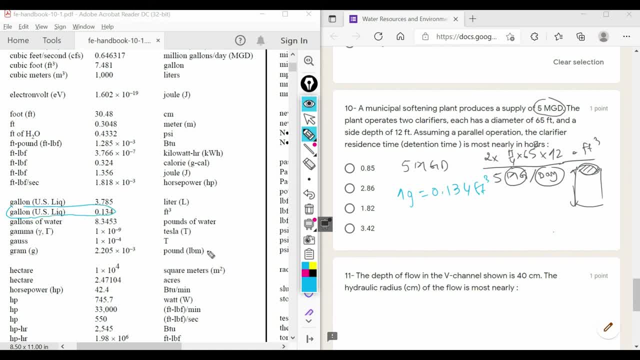 foot cube, foot cube. okay, so this is the formula here. so what? okay, so this is the formula here. so what? okay, so this is the formula here. so what we need to you, we need to you, we need to you to do is just to plug and chug using these. to do is just to plug and chug using these. to do is just to plug and chug using these conventions, and we, we know that one day conventions and we, we know that one day conventions, and we, we know that one day is equal to, is equal to. 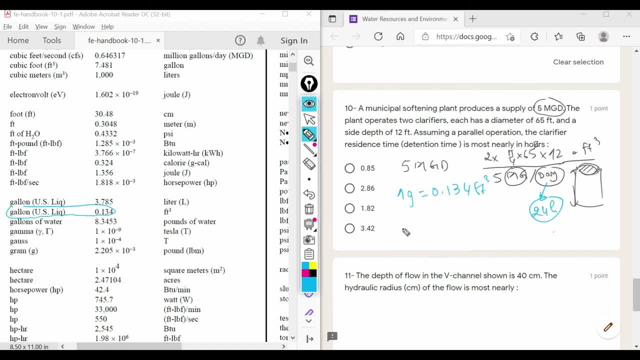 is equal to for 24 hours. so now the for 24 hours, so now the for 24 hours. so now the final result will be 2 multiplied by. final result will be 2 multiplied by. final result will be 2 multiplied by this value here p. 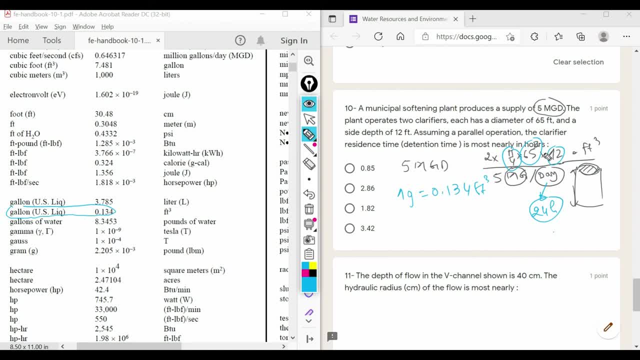 this value here: p. this value here: p: 5 square multiplied by 12. 5 square multiplied by 12. 5 square multiplied by 12. multiply by uh: nothing. so divide by multiply by uh: nothing. so divide by multiply by uh: nothing. so divide by uh. 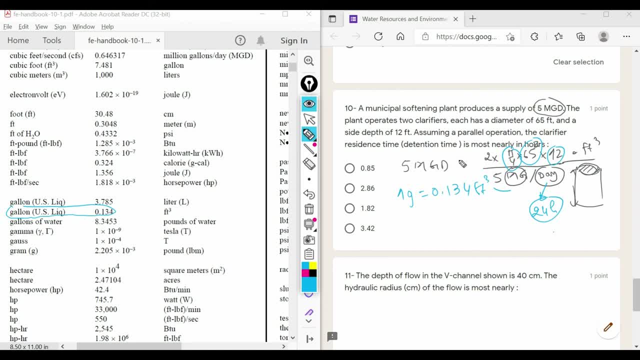 uh, uh, five, five, five. multiply by million, which is 10, power 6. multiply by million, which is 10, power 6. multiply by million, which is 10, power 6, so million. here is 10 to the sixth power. so million. here is 10 to the sixth power. 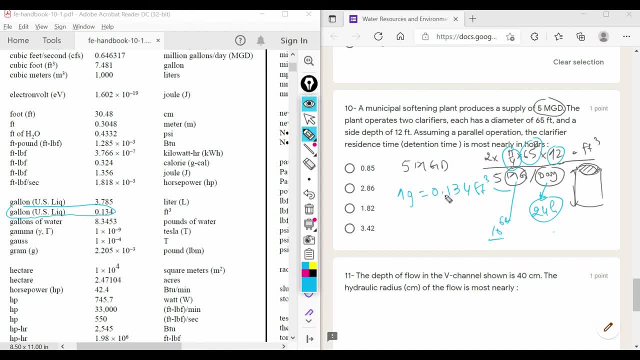 so million. here is 10 to the sixth power, multiplied by one gallon, which is multiplied by one gallon, which is multiplied by one gallon, which is 0.134, 0.134, 0.134, and the final result we multiply by one and the final result we multiply by one. 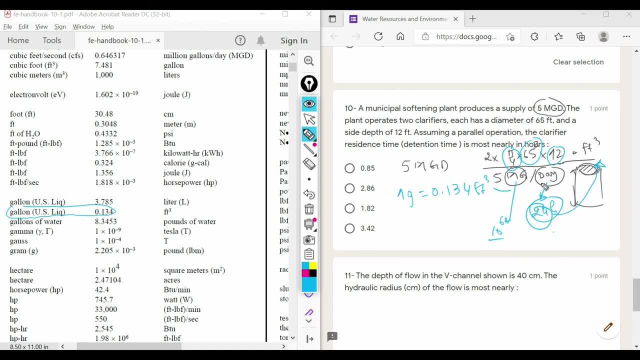 and the final result: we multiply by one: uh by 24, so 24 will come here. because uh by 24, so 24 will come here. because uh by 24, so 24 will come here. because 1 over 24 is this volume multiplied by. 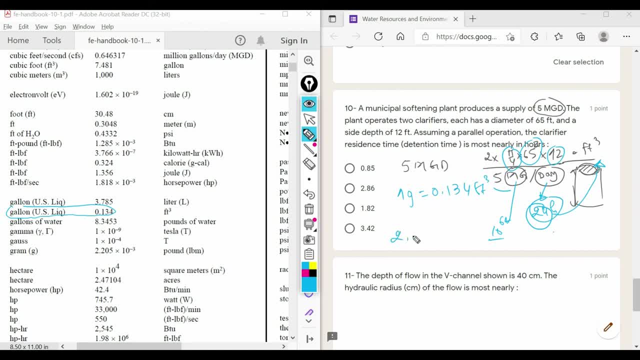 1 over 24. is this volume multiplied by 1 over 24? is this volume multiplied by 24, 24, 24, and finally we will find 2.853, and finally we will find 2.853, and finally we will find 2.853, which is very close to this value here. 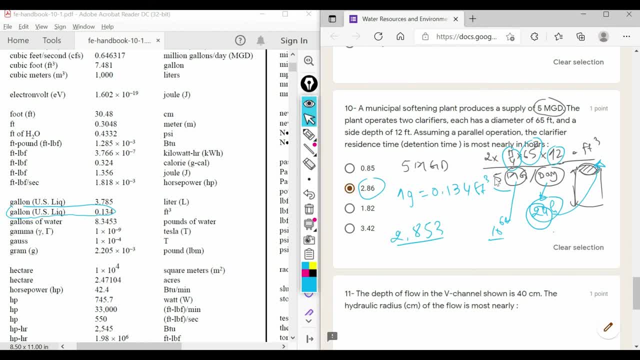 which is very close to this value here, which is very close to this value here. so, uh, this is a good answer. but so, uh, this is a good answer. but so, uh, this is a good answer. but, uh, if during the exam you find some. uh, if during the exam, you find some. 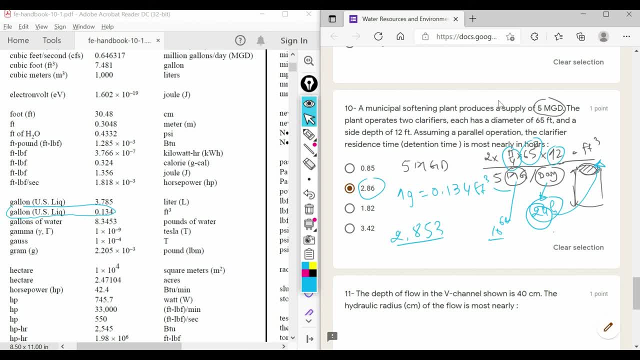 uh, if during the exam, you find some questions but you have no idea about how questions, but you have no idea about how questions, but you have no idea about how to solve them, the first thing to do is a to solve them, the first thing to do is a. 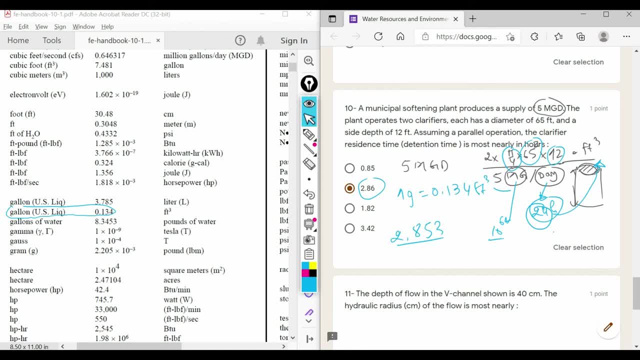 to solve them. the first thing to do is a dimensional analysis. this is a volume dimensional analysis. this is a volume dimensional analysis. this is a volume per time, and this is this, this per time, and this is this, this per time, and this is this, this information and this information will. 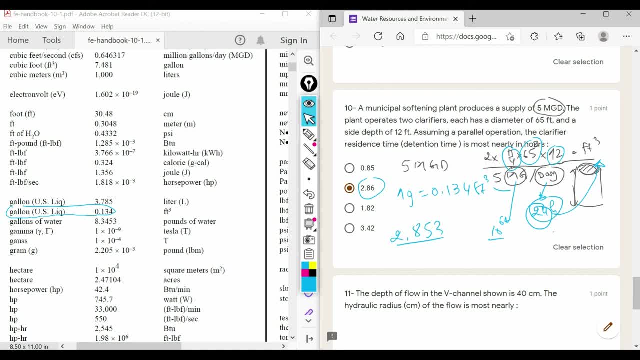 information and this information will information and this information will gives us the volume. so if you divide the gives us the volume. so if you divide the gives us the volume. so if you divide the volume over the volume over time, you, volume over the volume over time, you. 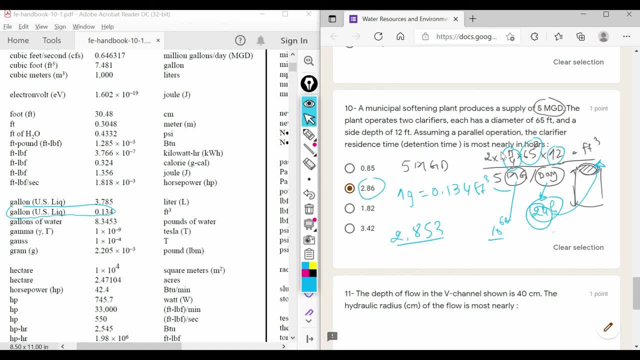 volume over the volume over time. you will have the time, will have the time, will have the time, and and and there will be uh some questions. there will be uh some questions. there will be uh some questions that are related to common sense, even if that are related to common sense, even if 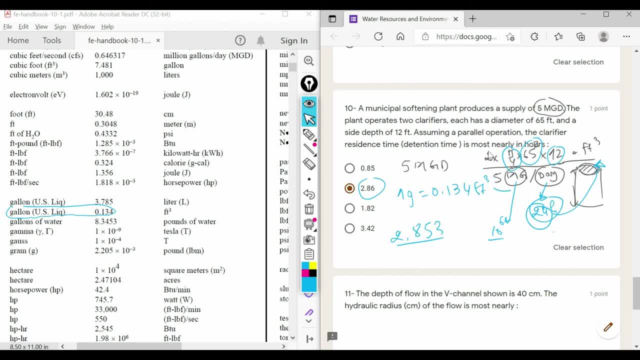 that are related to common sense. even if you don't know how things, you don't know how things, you don't know how things function, just try to guess how to use function. just try to guess how to use function. just try to guess how to use the dimensional analysis to find an. 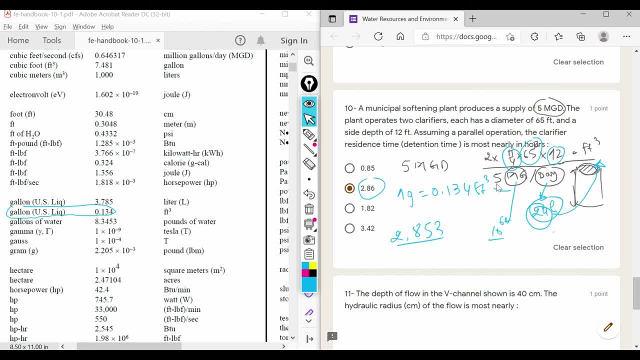 the dimensional analysis to find an. the dimensional analysis to find an answer, and your guess will be more answer, and your guess will be more answer and your guess will be more: uh, reliable than just guessing. uh, reliable than just guessing. uh, reliable than just guessing using 25. 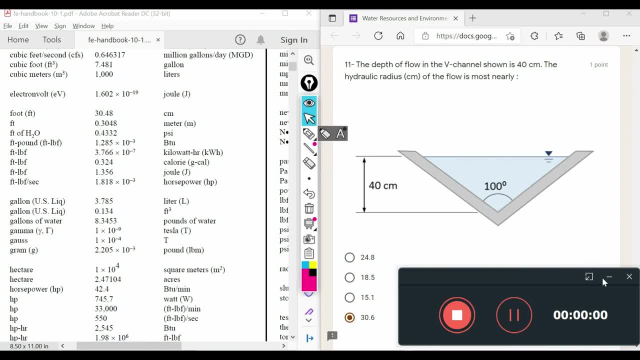 using 25. using 25, chance of having the good answer, chance of having the good answer, chance of having the good answer. so the final question is about the. so the final question is about the. so the final question is about the hydraulic radius. again, hydraulic radius, again. 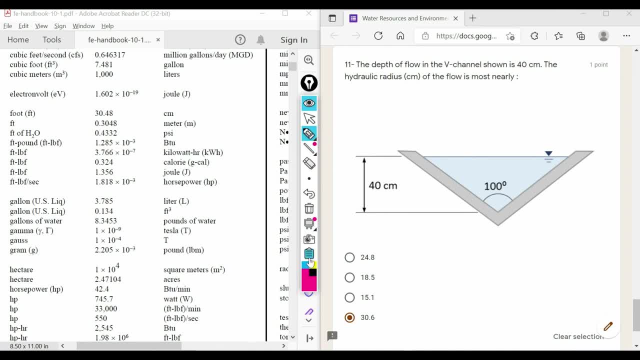 hydraulic radius again, and this time is a little bit tricky, but, and this time is a little bit tricky, but, and this time is a little bit tricky, but the same concept applies here again, the same concept applies here again, the same concept applies here again. so we have hydraulic radius is the 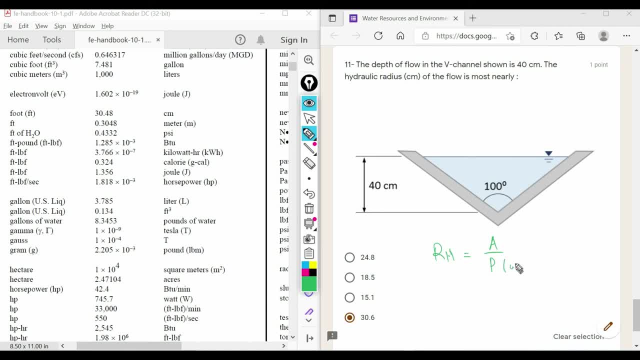 so we have hydraulic radius. is the- so we have hydraulic radius. is the cross-sectional area over the weighted cross-sectional area, over the weighted cross-sectional area, over the weighted parameter. so it's the weighted parameter, so it's the weighted parameter, so it's the weighted parameter. 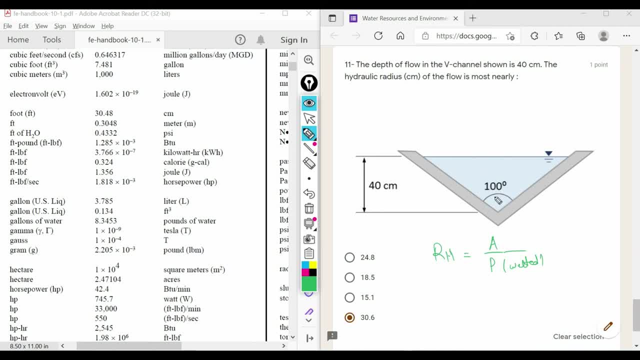 parameter, parameter, but first we need to, but first we need to, but first we need to find, find, find some values here, because we only have some values here, because we only have some values here, because we only have this height, this height, this height which is equal to 40 centimeters. so we 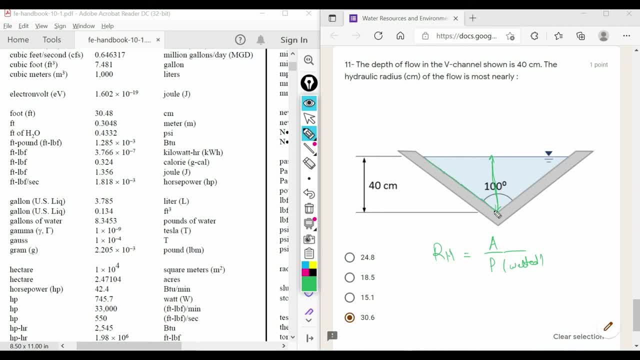 which is equal to 40 centimeters. so we, which is equal to 40 centimeters, so we need to find, need to find, need to find this distance here, this distance here, this distance here, and this and this and this distance here, so we have a symmetrical triangle about 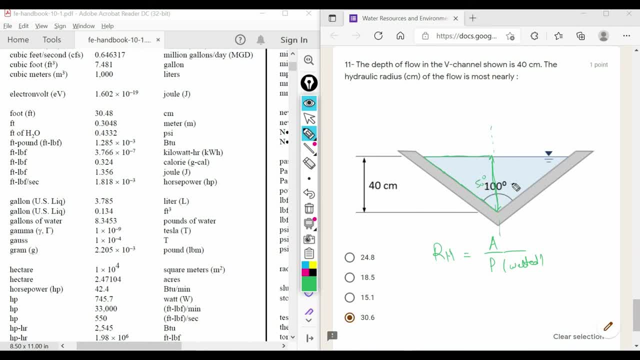 we have a symmetrical triangle about. we have a symmetrical triangle about this axis here. so here we'll have 50, this axis here. so here we'll have 50, this axis here. so here we'll have 50 degrees. you will have 50 degrees, so this. 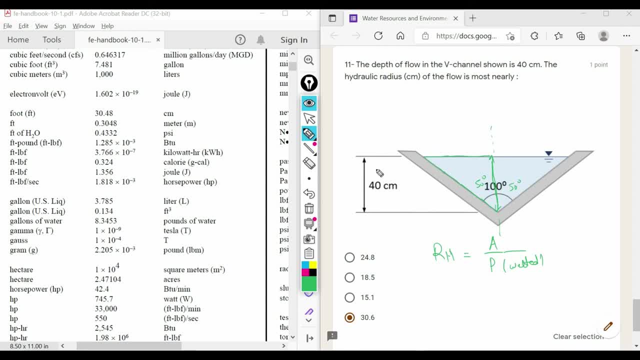 degrees: you will have 50 degrees. so this degrees: you will have 50 degrees, so this side here will be equal to side here will be equal to side here will be equal to the height which is equal to 30. the height which is equal to 30. 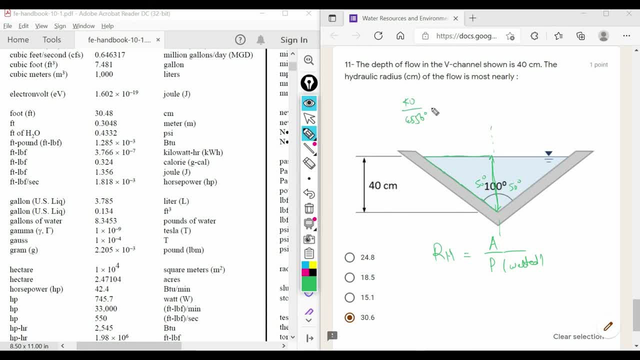 the height, which is equal to 30 centimeters over cosine of 50 centimeters over cosine of 50 centimeters over cosine of 50, so will be equal to: so will be equal to, so will be equal to 40 over cosine 50, 40 over cosine 50. 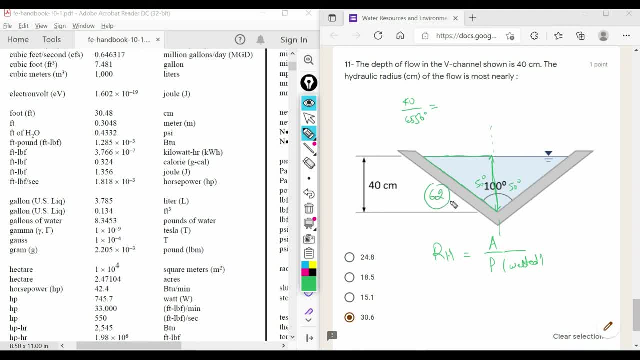 40 over cosine 50, which is equal to 62, which is equal to 62, which is equal to 62 centimeter, centimeter, centimeter, and this one, you can find that you and this one, you can find that you and this one, you can find that you, using the, 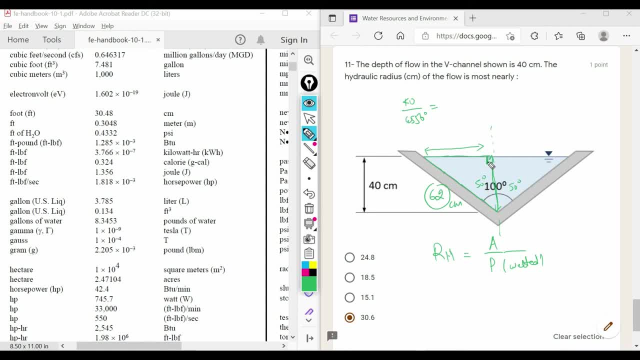 using the tangent or using the. we have using the tangent or using the. we have using the tangent or using the. we have here a, here a, here a square triangle. so this is equal to square triangle. so this is equal to square triangle. so this is equal to square root of 62. 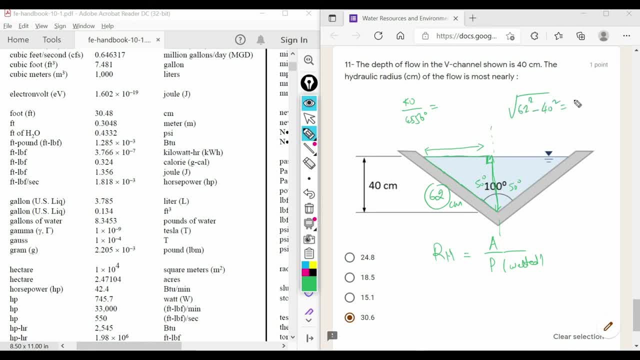 square root of 62, square root of 62 square minus square, minus square minus 40 square, which is equal to 74.37. so now let's 74.37. so now let's 74.37. so now let's uh, uh, uh, let's find our. 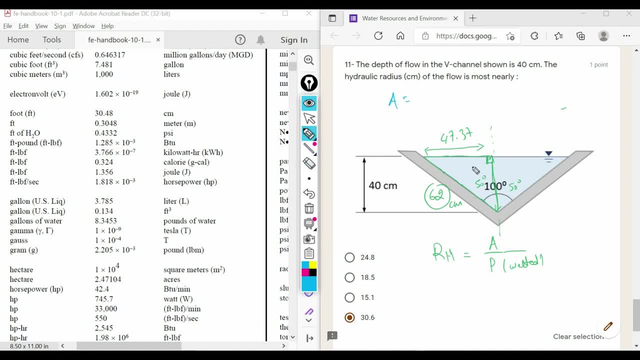 let's find our, let's find our, our area. so the area here is equal to our area. so the area here is equal to our area. so the area here is equal to the area of this triangle, the area of this triangle, the area of this triangle, all of this area here, which is equal to. 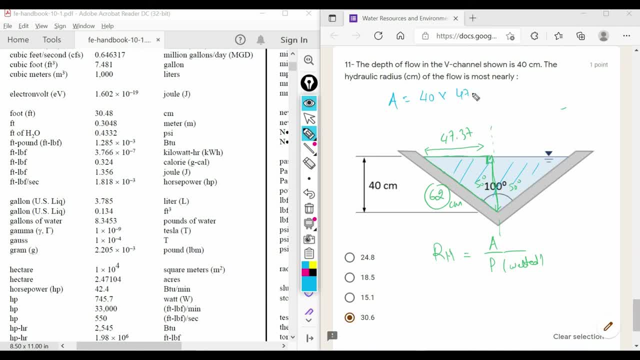 all of this area here, which is equal to all of this area here, which is equal to the height, the height, the height. multiply by this one, multiply by this one, multiply by this one, multiply by two in order to have the space, multiply by two in order to have the space. 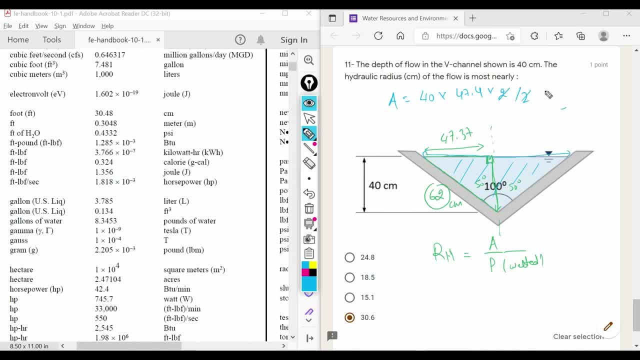 multiply by two in order to have the space here, from here to here, here from here to here, here from here to here, over two over two, over two, so, which is equal to so, which is equal to so, which is equal to 40 multiplied by 47.4. 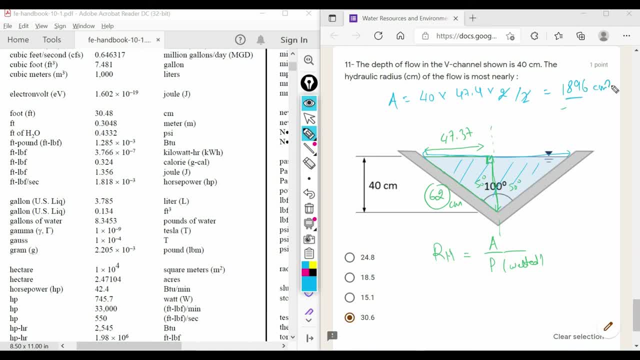 40 multiplied by 47.4. 40 multiplied by 47.4 is equal to 1: 8 is equal to 1. 8 is equal to 1: 8 centimeter square. and now the perimeter. centimeter square. and now the perimeter. 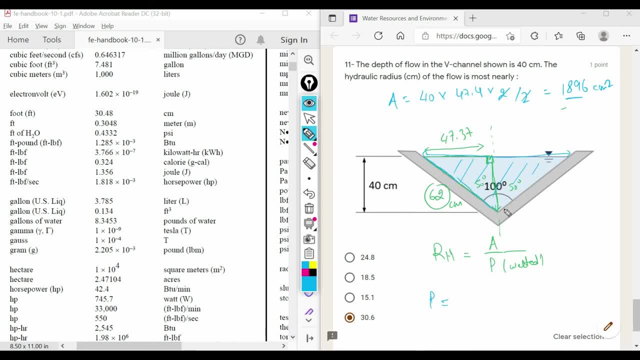 centimeter square. and now the perimeter you have to pay attention is equal to you have to pay attention is equal to you have to pay attention is equal to this side, this side, this side plus this side, so we don't have you plus this side, so we don't have you. 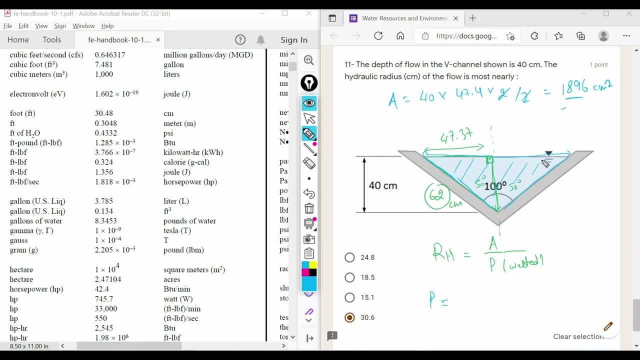 plus this side. so we don't have, you don't have to include the base. because don't have to include the base, because don't have to include the base? because the bait is not awaited, the bait is not awaited. the bait is not awaited. it's not a weighted perimeter, so it's 62. 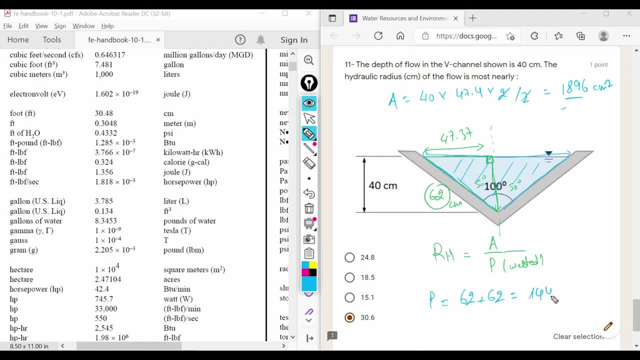 it's not a weighted perimeter, so it's 62. it's not a weighted perimeter, so it's 62 plus 62, which is equal to plus 62, which is equal to plus 62, which is equal to one, four, four and finally, if you plug,